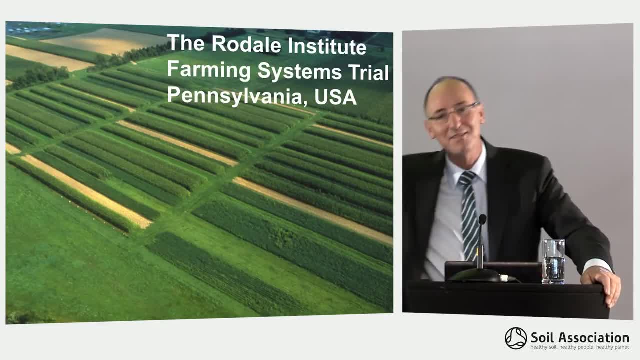 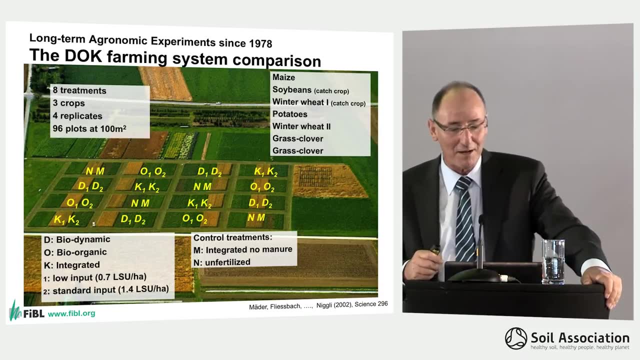 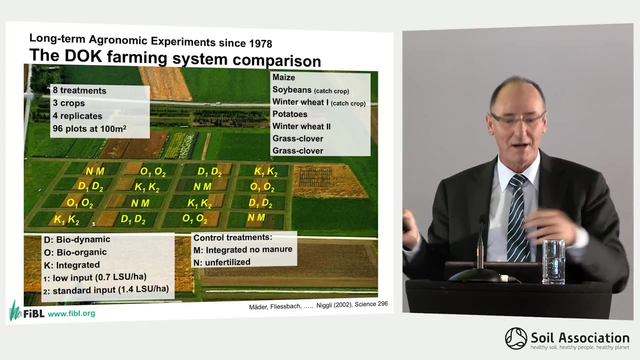 that the Rodale data is always on one side, on the very optimistic side and on the very optimistic side, And I will also use data, for instance, from our DOC farming trial in Switzerland, in the northern part of Switzerland, where we compare different farming systems. 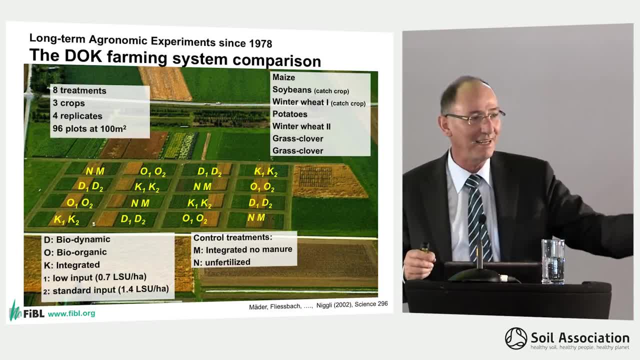 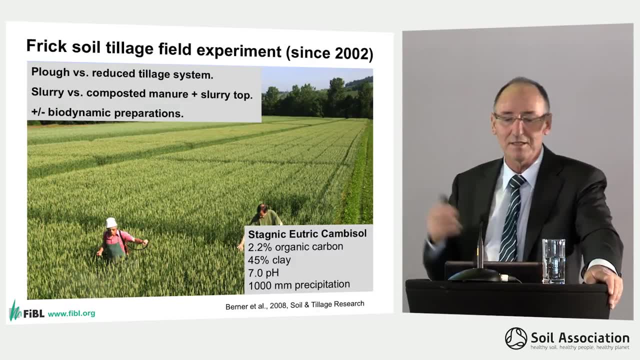 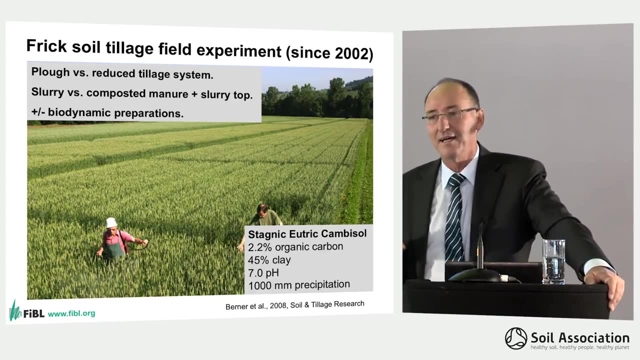 and this is always on the careful side of the data. But then we also have other experiments in Switzerland, for instance about organic soil tillage, where we use the same data to see if the soil is reduced or minimum till. Is that possible? 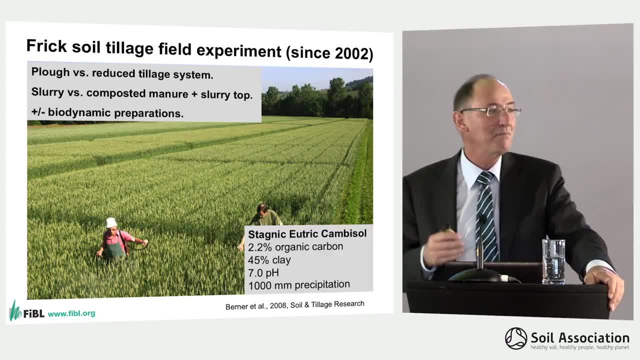 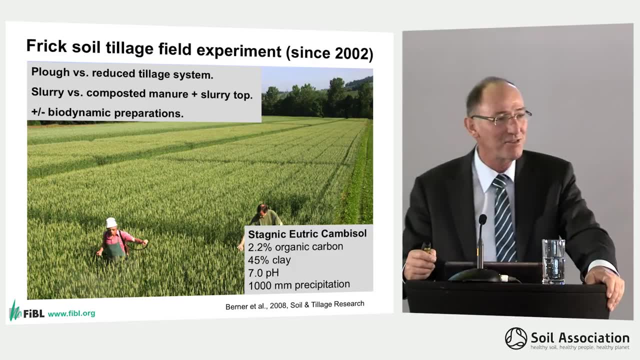 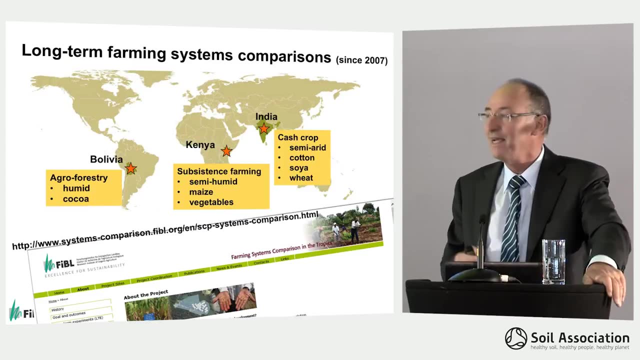 to be combined with organic farming. Peter Melchatt always says: don't promote that because it's too dangerous for organic farmers. But you'll see that we do that in a quite successful way And we also started a few years ago with long-term farming system comparison in: 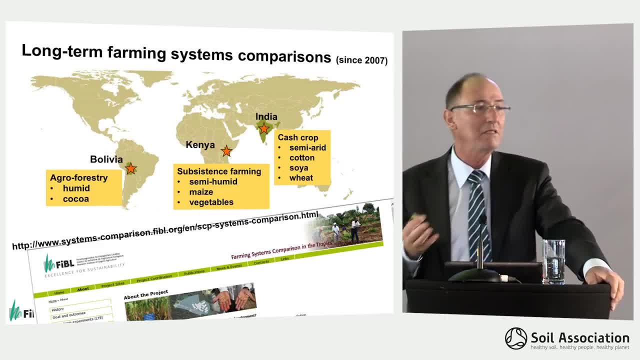 in the tropics, because there is almost no data available on organic farming in tropical soils, and this is crucial to have more information about that, because the future of organic also lay in tropical countries and not only in temperate zones. So we have established a few. 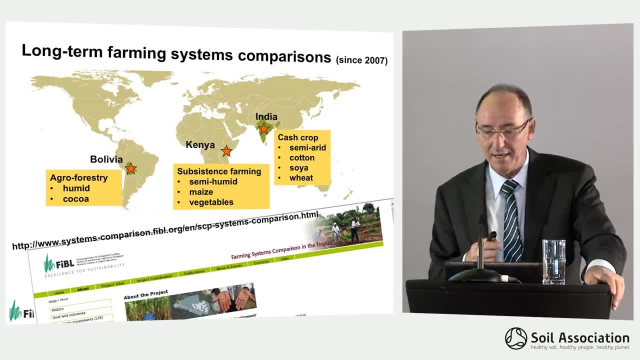 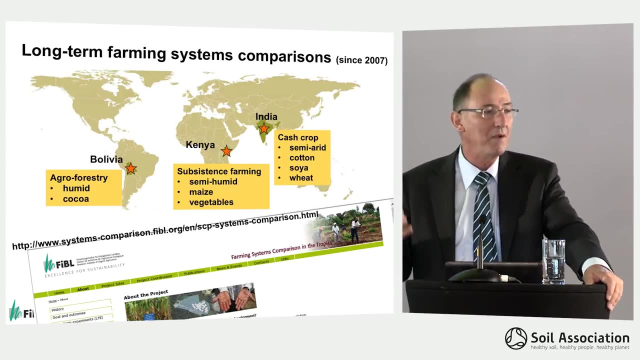 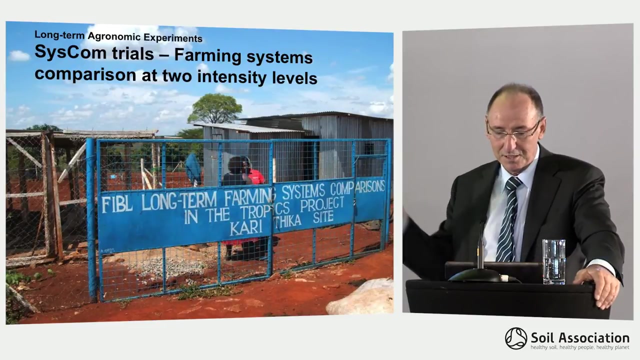 years ago in Bolivia and Kenya and in India, long-term comparison trials in a totally different context, with totally different crop rotation, but with always the same question: how does organic perform compared to GMO, to conventional farming and to other subsistence farming systems which are locally represented? So this is the one in Kenya, one of our farms. 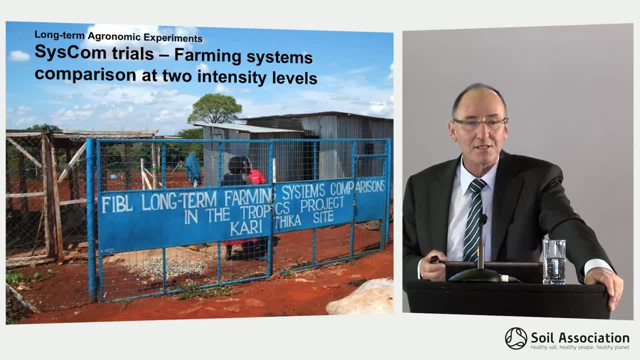 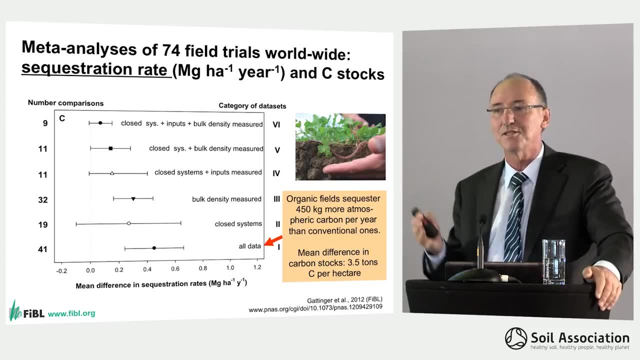 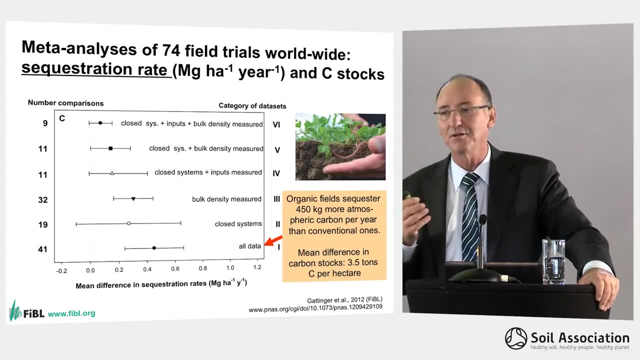 in the, in the research sites there. So I'm going to show you now some results, because it's important as an organic farmer to know where does organic farming really perform better than conventional farming, because otherwise, if we won't perform better, it doesn't make sense that we farm in such a complicated way. 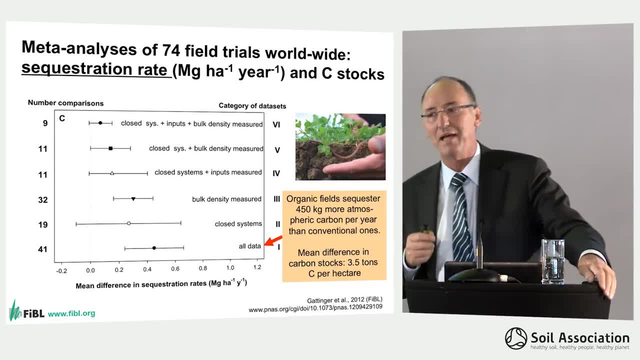 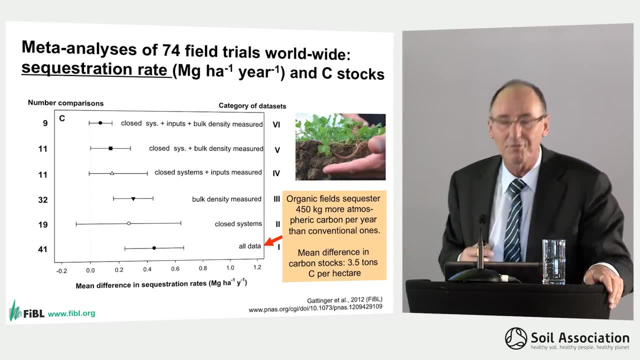 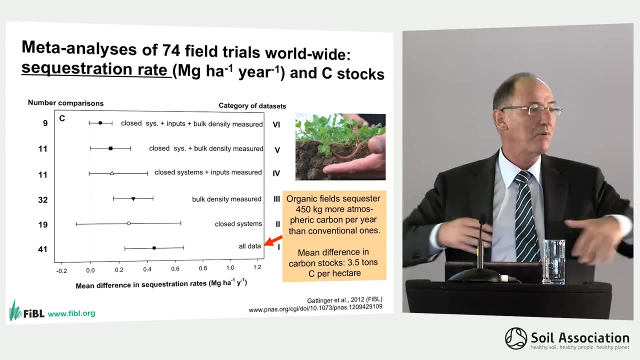 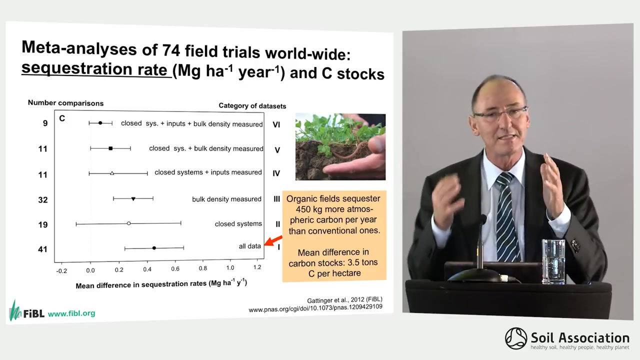 So it has to, we have to perform better, and this is data from this META, global META analysis and we received from all these 74 long-term field trials all the raw data that they produced over many, many years and we calculate it then once again to really to have a statistical, a scientific overview on 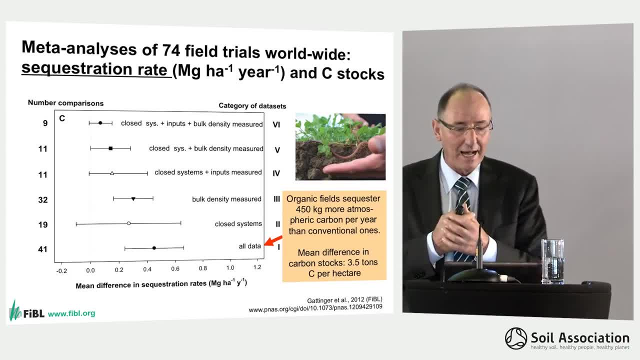 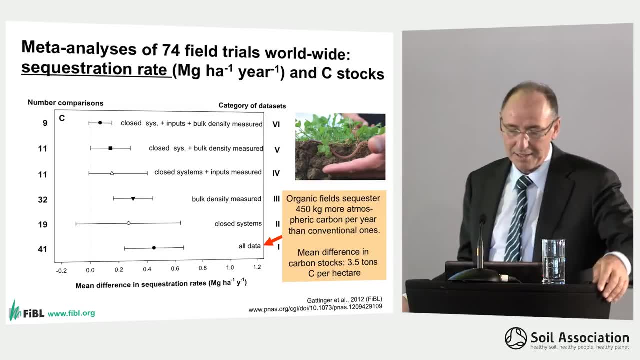 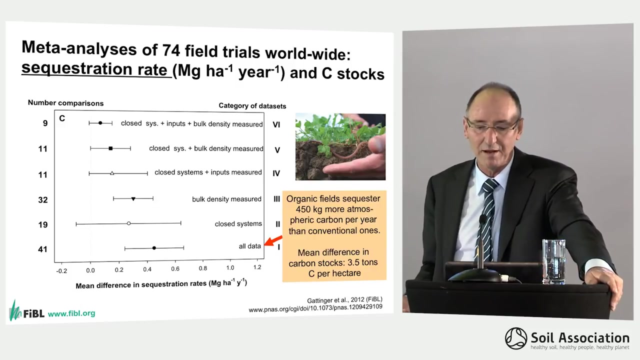 the outcome of all the data Aand the most. The most important result is- and this was published in the Proceedings of National Academy of Science in the United States, one of the most prestigious scientific journals. So the most important information I can give is that organic fields sequester 450 kilograms more atmospheric carbon per year than conventional ones. 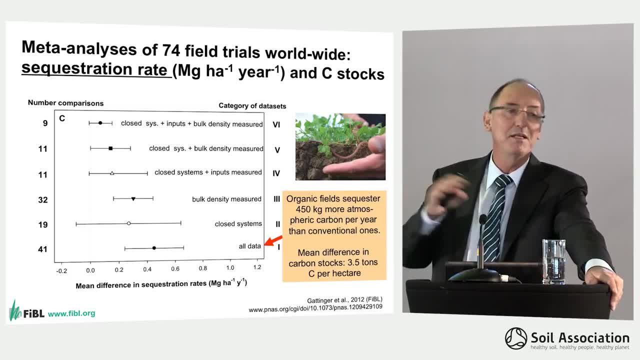 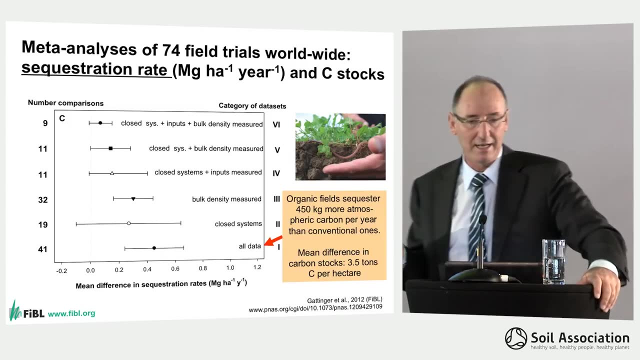 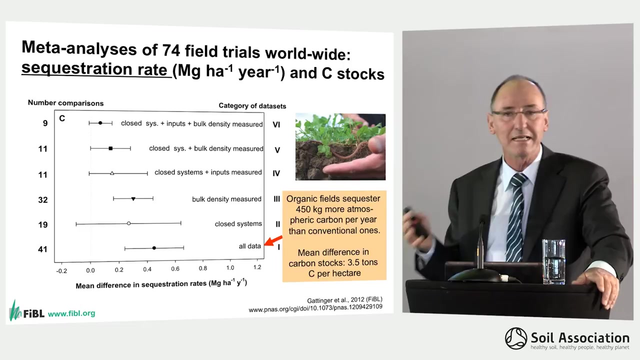 And the mean difference in carbon stocks between conventional and organic fields is 3.5 tons carbon C per hectare. So this is A Average data from all these 74 long-term field trials, and the mean duration of these field trials is 16 years. 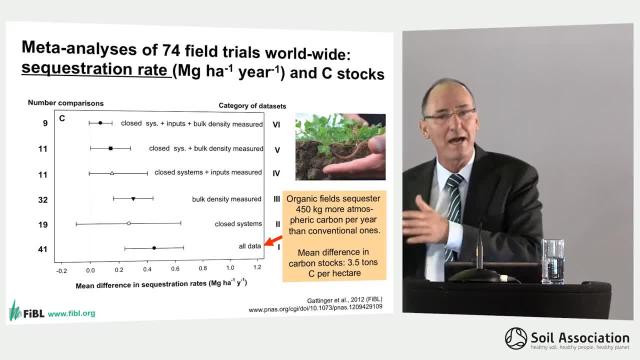 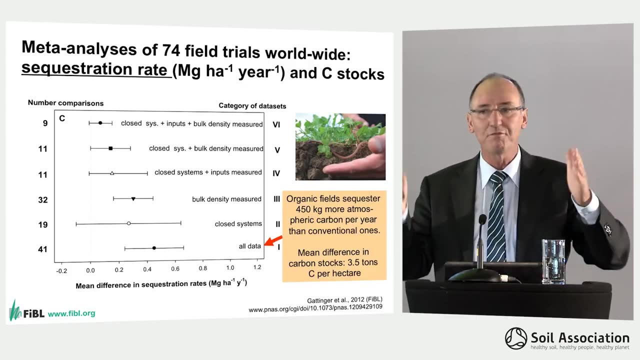 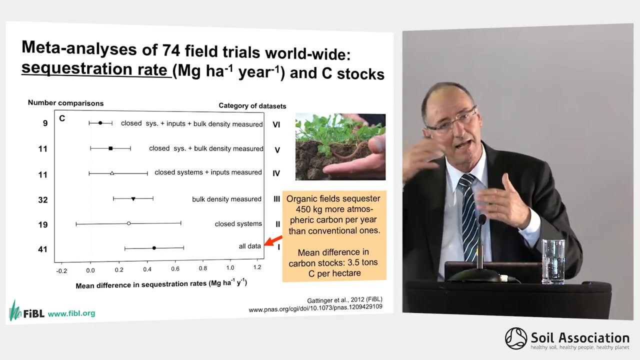 And so it's not a short impact a short effect, it's really a long-term effect And we see in many of the very old long-term comparison trials that the sequestration of carbon if you have different, If you have different farming systems and if you convert to organic, it is a long-lasting effect. You can count that it lasts at least 20, 25 years. In Scandinavian soils they even saw this sequestration by organic farming lasting for 50 years. Of course these soils in the north are not so fast digesting organic matter. 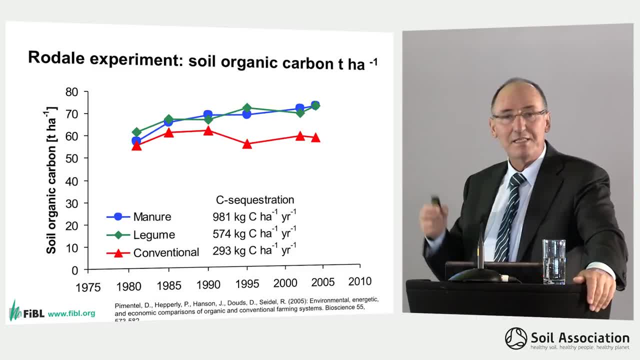 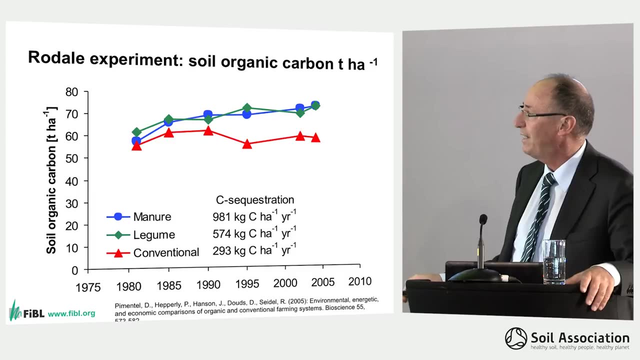 And you see these differences in conventional and organic farming Also in the single experiments. here is again the Rodale experiment where you can see the sequestration rates, The two organic systems with manure and legume and the conventional system. So the conventional system is quite stable. 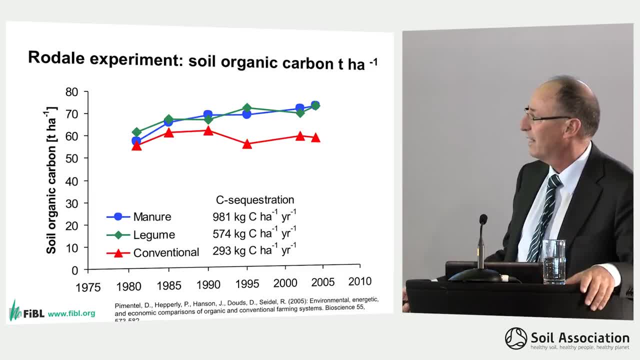 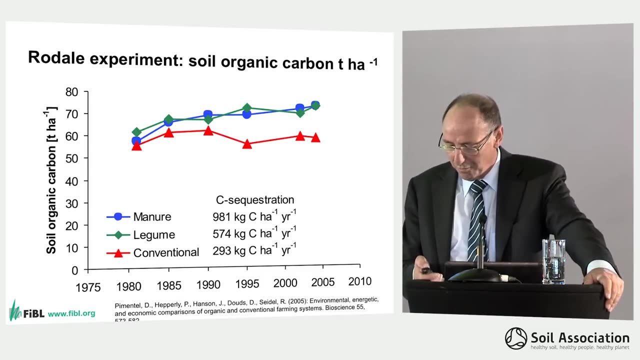 And the sequestration rate drops rates are at about 300 kilogram C per hectare and year And the manure system goes up to almost 1,000 kilogram carbon per hectare and year. For me, this is a little bit this. 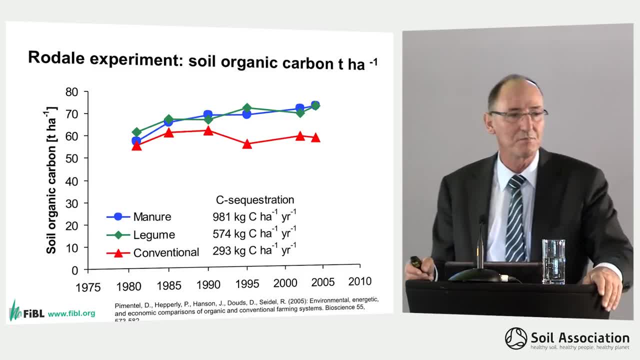 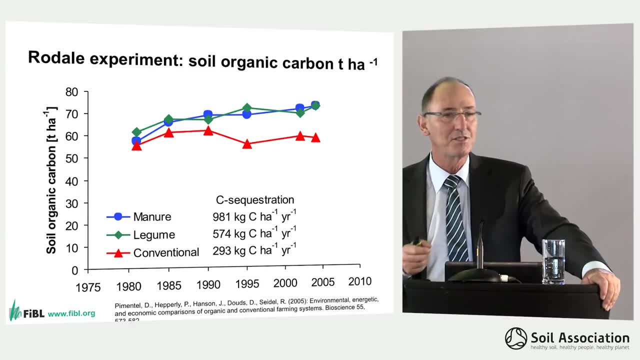 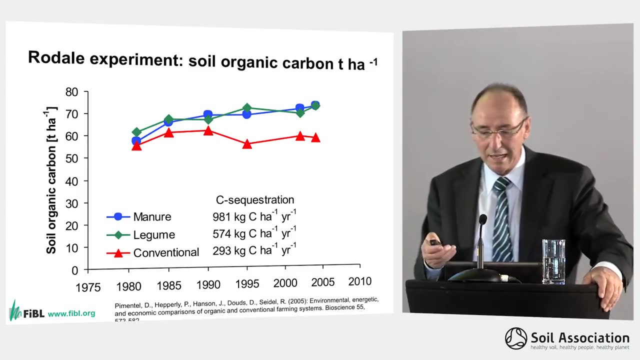 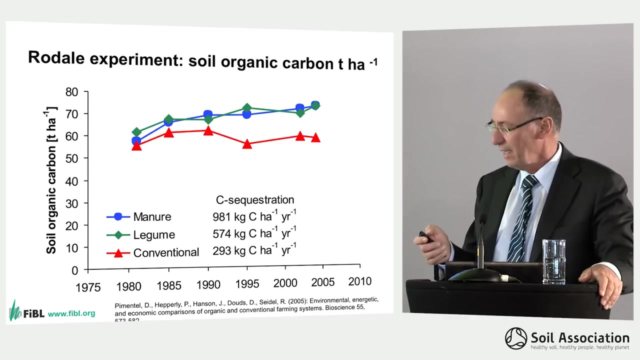 is not representing an average farming system, because they put a lot of organic manure and of organic material into the soil And this is not representing the daily practice of organic farmers, But nonetheless, you see what is possible as sequestration rates when you farm with manure, with legumes and so on. 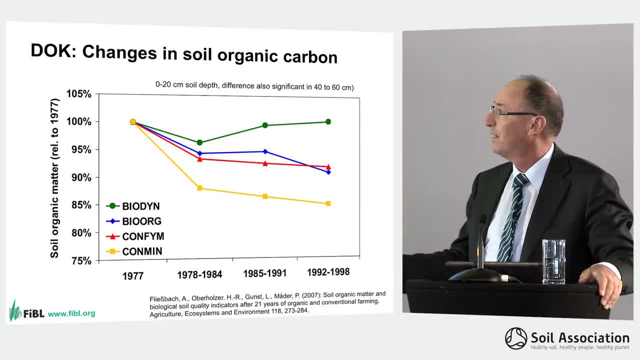 A little bit the same situation we have in our Swiss dog trial. You see that the biodynamic system has remained quite stable, although the crop production, The crop rotation, is a very intensive one, with a lot of wheat in the rotation, And it is increasing now. 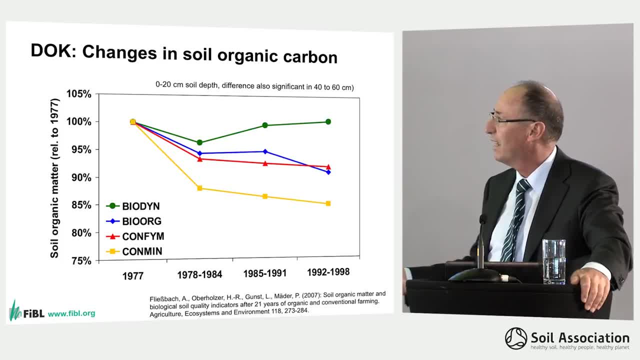 And it has increased further in the last years And you see that the very conventional farming system, without any manure, only mineral fertilizer. they have lost already 15% of the carbon which was there at the very beginning of the trial. 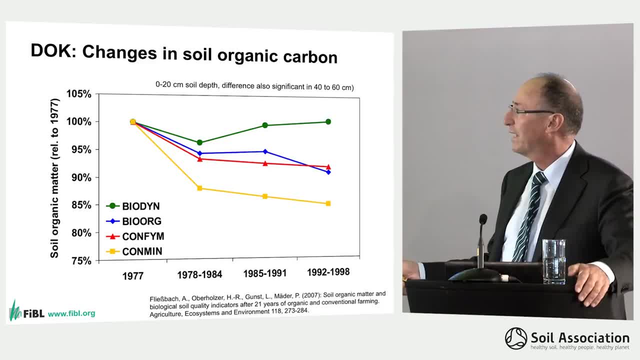 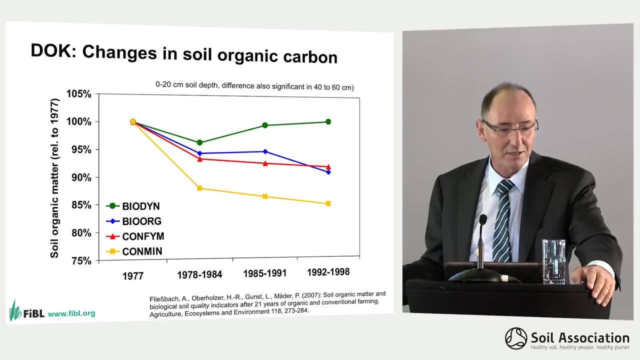 And you can see that both organic with manure and integrated with manure have almost the same values. So it's really the manure, the recycling, which is relevant, And it's not so much whether you believe into an organic or a conventional god. 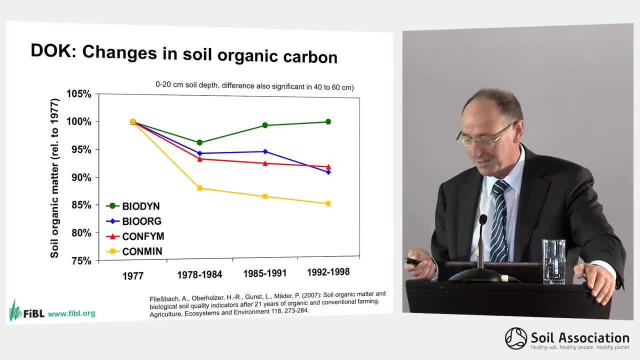 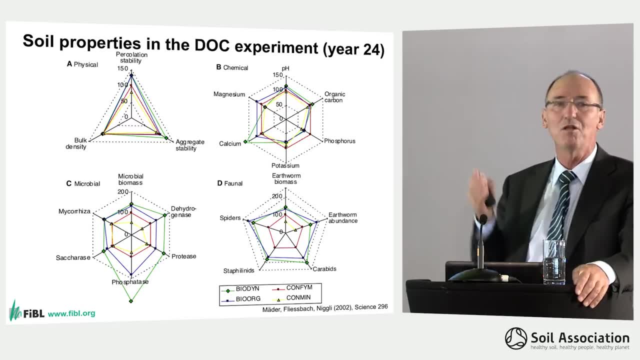 So it has its clear scientific reasons. What was really amazing when we looked at it? we looked into all kinds of soil properties in this very dog trial in Switzerland- that you cannot see the details. But what we can see is that the physical properties of soil 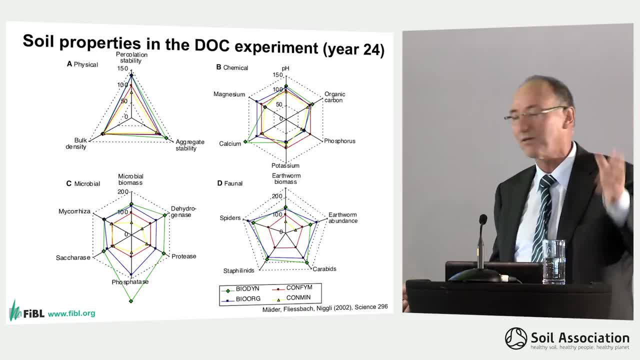 the two organic systems, the biodynamic and the conventional one were far better than the integrated. biodynamic and organic was far better than the integrated systems in physical properties, but also in the microbial properties. Some enzymes were double or triple the concentration in soils. 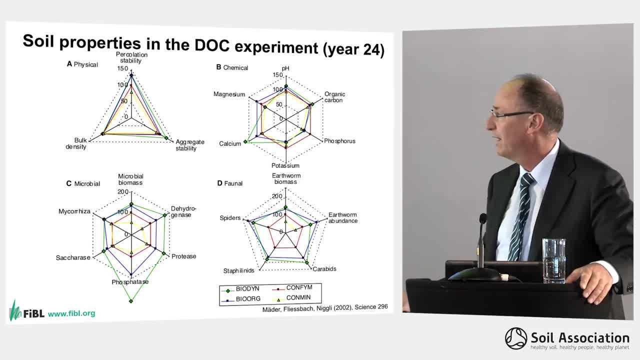 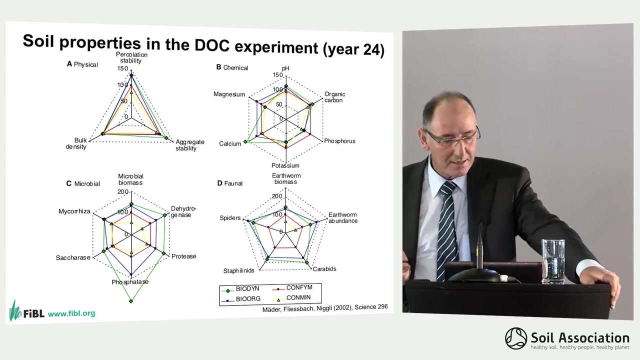 than in conventional farming systems, But also in soil, fauna, earthworms, spiders, caribbits, biomass and so on, It was much better the organic systems than the conventional one. This was all published in Science in 2002.. 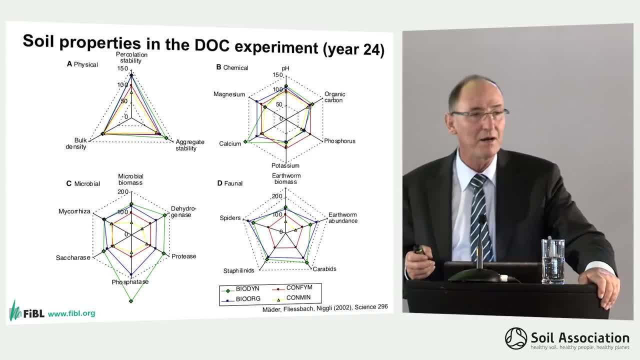 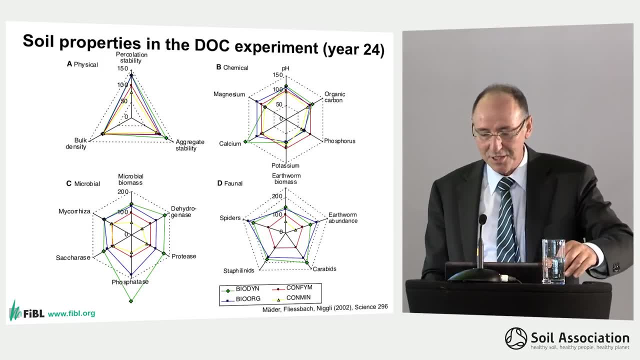 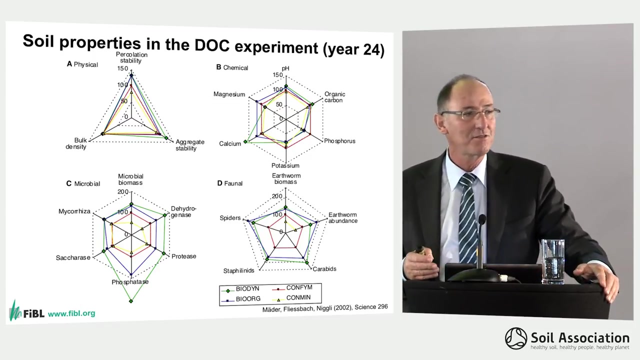 And when we published it we were very much attacked by many of the conventional of the GMO people who campaigned For GMO and we delivered a lot of scientific data to all these peoples, especially from the United States And finally, for instance, from Mr Avery Junior. 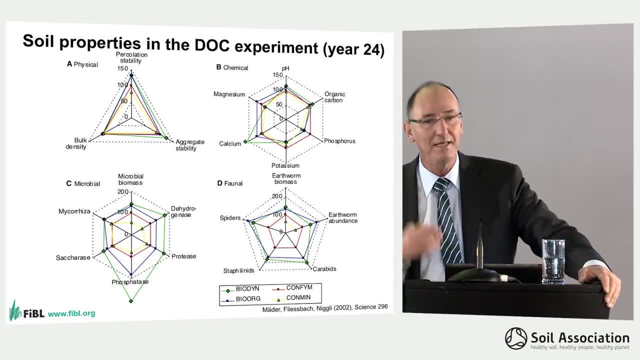 who was at that time very aggressively campaigning against organic, in favor of the GMO industry. he came back with the answer. unfortunately, I couldn't find any fault in your answer Because of the fact that I have a very good knowledge about organic in the environment and the way. 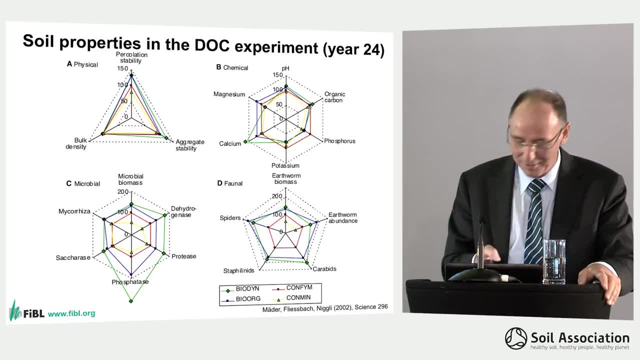 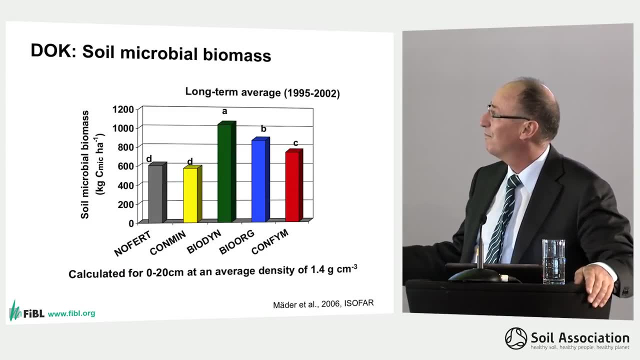 you do your analysis, your conclusions, I have to accept that your conclusions are scientifically sound. For me, that has been so far the biggest compliment I've ever received. You can see, looking, for instance, at soil, microbial biomass, the biodynamic 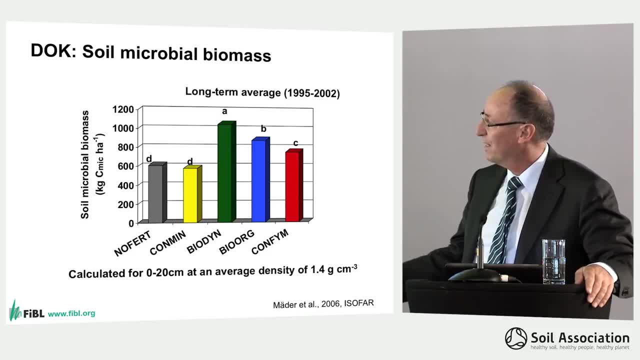 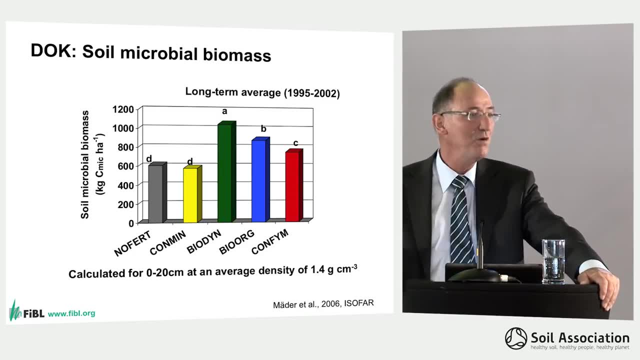 ones are always better than the conventional ones and you can see if you have a very good integrated production with a lot of manure you can come a little bit closer to organic. but you cannot be as good as organic because also the pesticides you use have an influence. 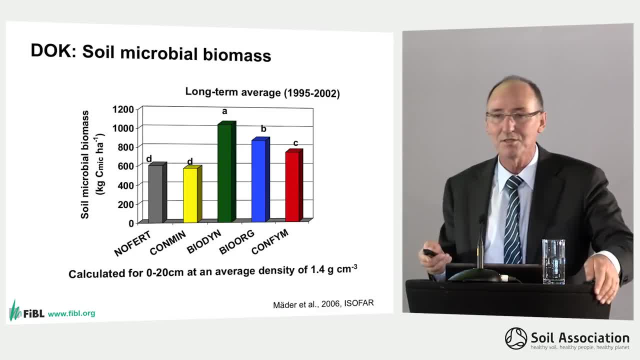 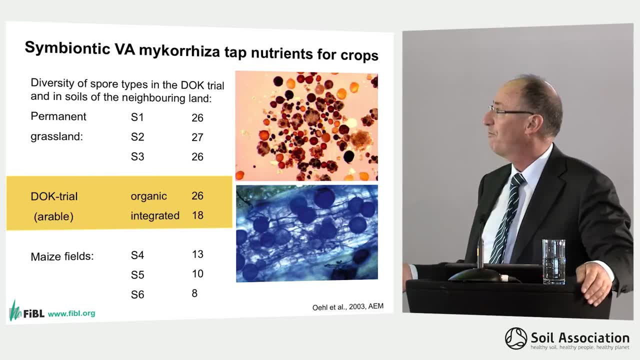 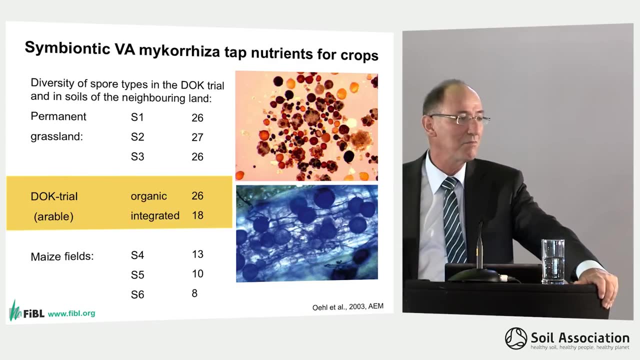 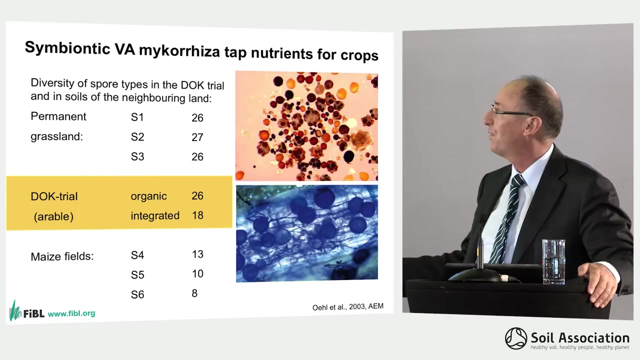 on soil, biomass and on all the animals living in the soil. what is really fantastic was that we saw differences really down to the diversity of microorganisms and microorganism functions in the soil, for instance mycorrhizae, which are extremely important because they can tap. 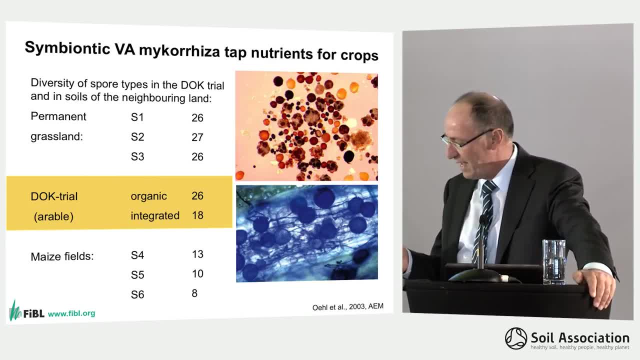 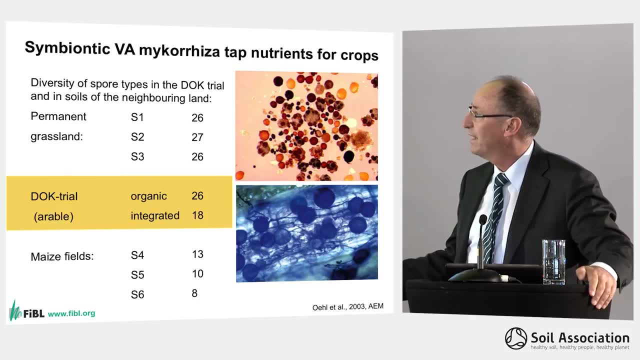 nutrients for crops, especially phosphorus. and you can see- look here these are the, the, the, the, the, the diversity in the number of different spore types we found in the organic and in the integrated fields of the dog trial. and you can see, this is what we found in the. 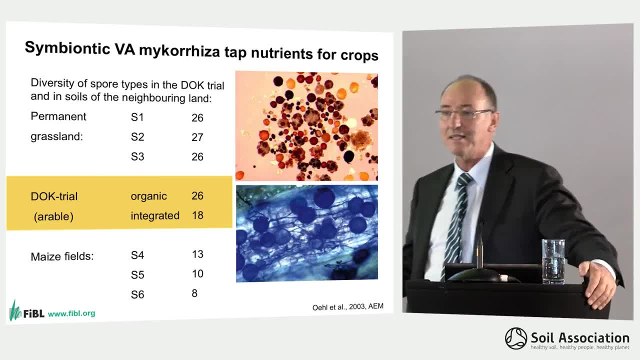 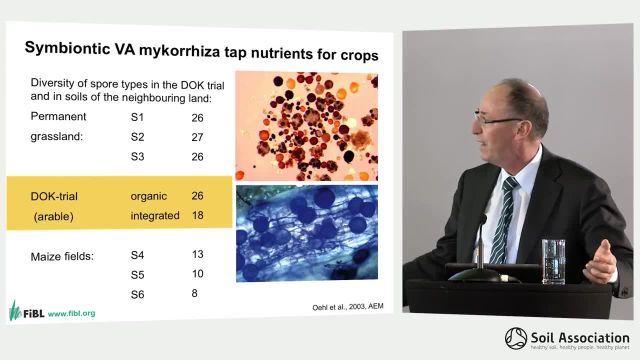 immediate neighborhood in permanent grassland which is always very rich in different spore types, and this was what we found in maize fields in the neighborhood, which are always a little bit poorer, and you can see that the arable fields of the dog trial organic are very 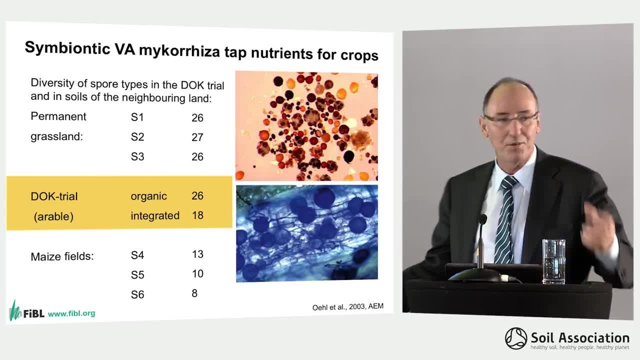 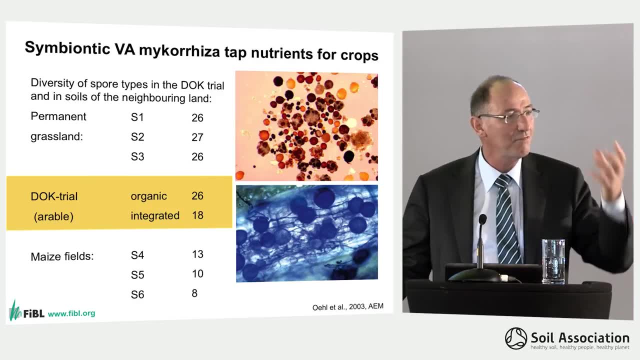 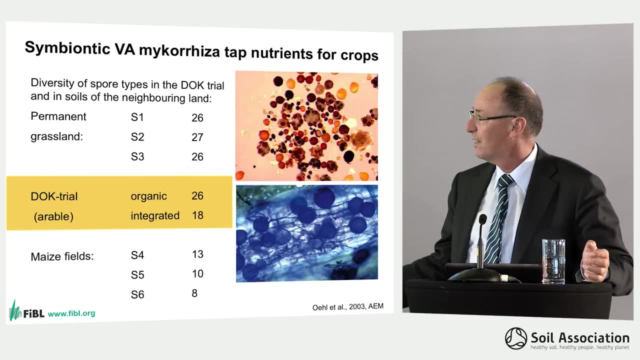 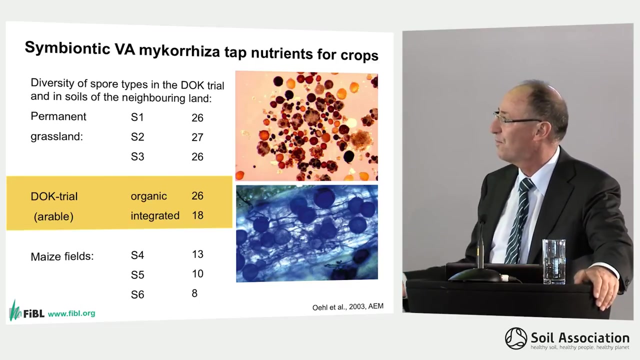 close to the high diversity of permanent grassland, even though it's it's it's it's plowed, even though it's intensively managed. so the diversity of of organic arable land looks, looks equal to the to high diversity sites on the permanent grassland and the. 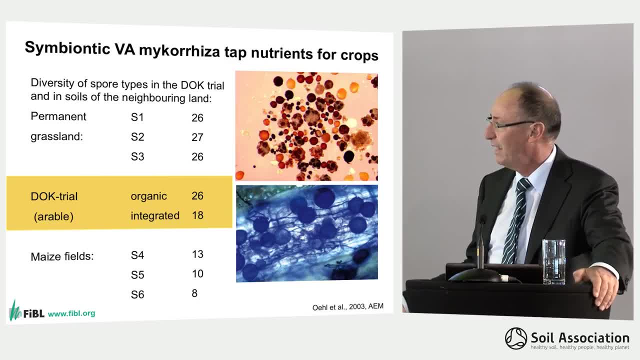 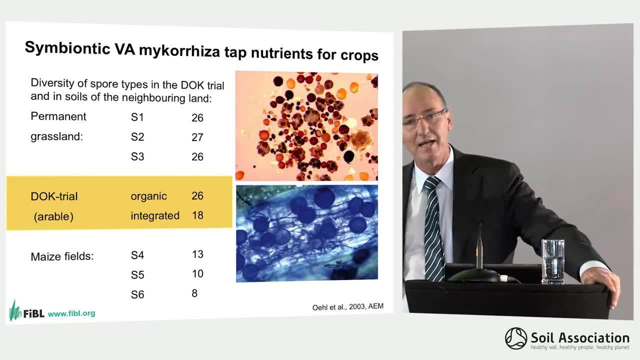 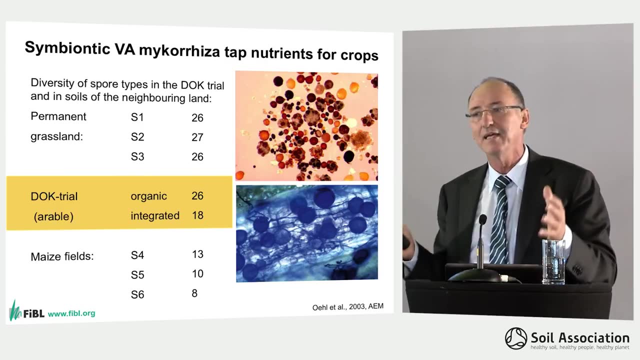 integrated farming system here of the dog trial is closer to maize fields in the neighborhood, so this, this is really a continuous trend. we can measure that we can keep, also under arable cropping, a high diversity in soil, and this is exactly what Helen mentioned. this is this. 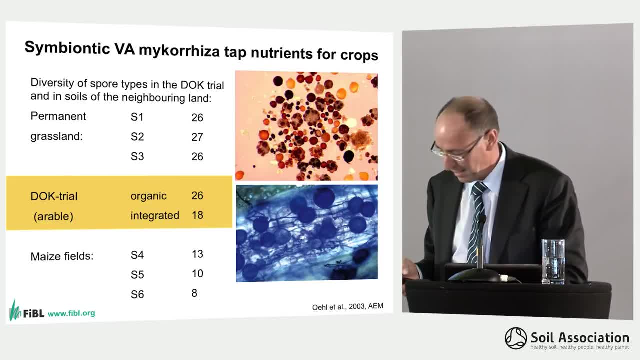 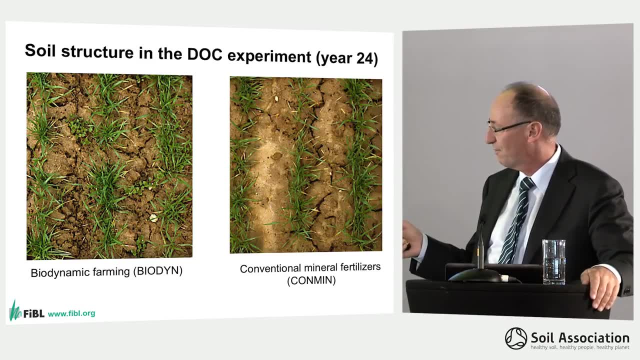 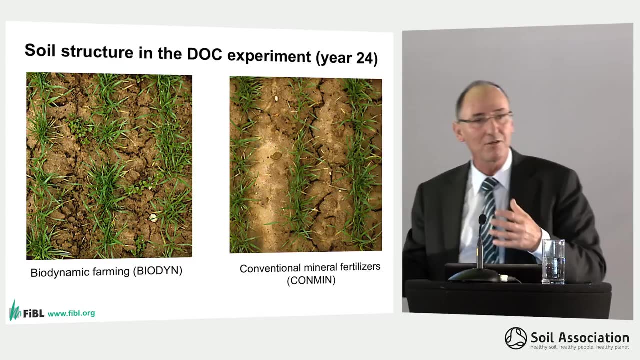 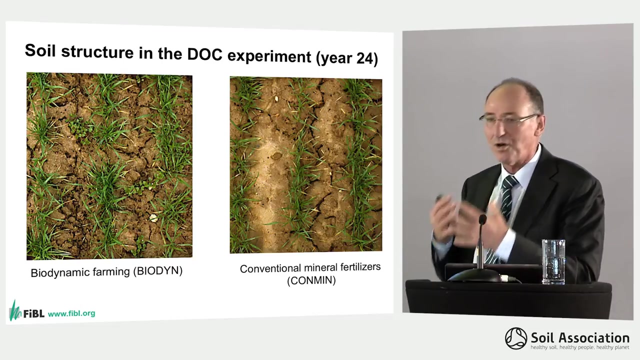 is really our wealth. we have in organic farming and did- some of you might already have seen these pictures at several times so and all what we can measure in soil diversity and in soil microbiology is is also can also be seen in soil structure, because so soil life. 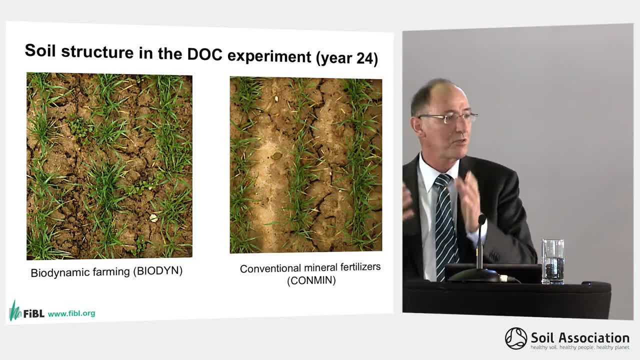 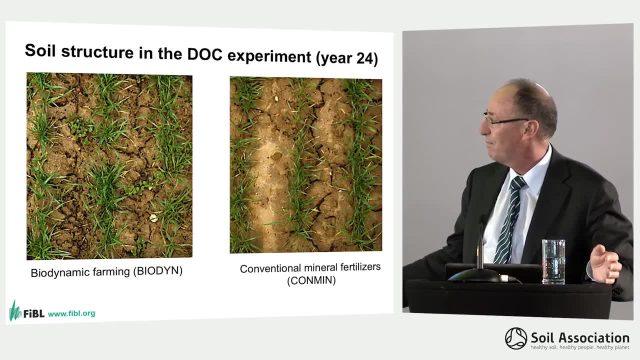 is very closely linked to soil structure and it's extremely important and you can see here that this is the biodynamic field in the year 24- winter wheat. this was in October or November of the year 24 of the crop rotation and you can see the difference here between conventional 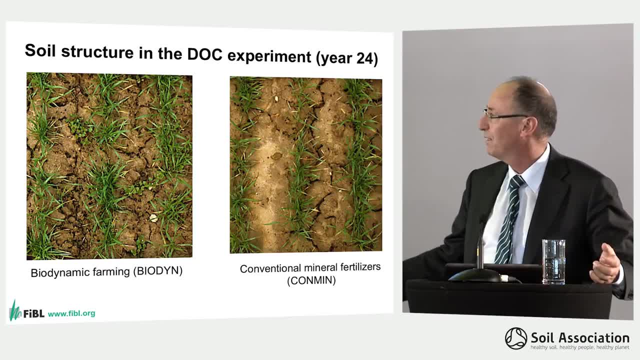 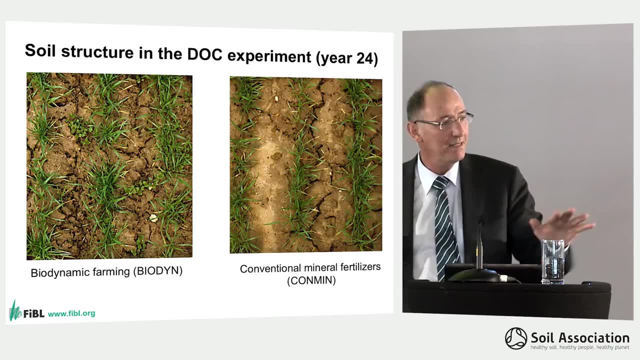 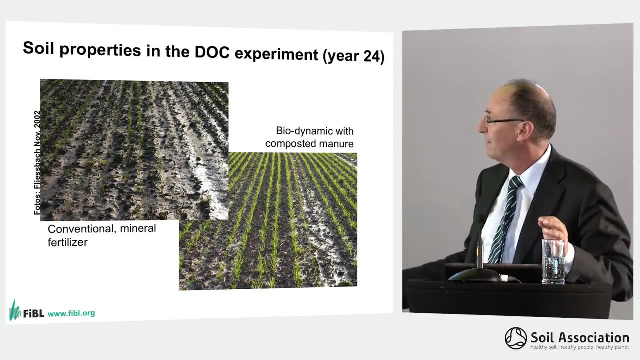 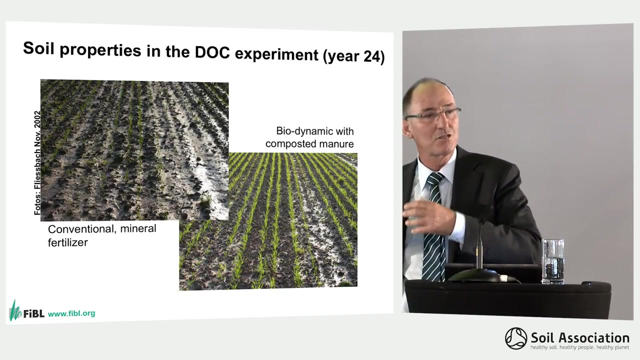 field, the conventional field, and the biodynamic field. it's a huge difference. the soils, the soil structure on the surface is completely different, and this you. the result is, after a heavy rainfall, that biodynamic soil can really take up the water immediately, can can store it and 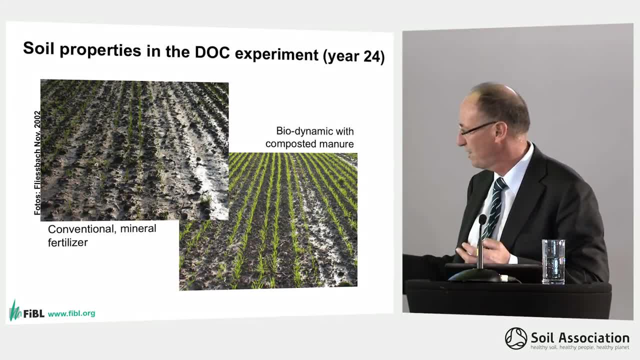 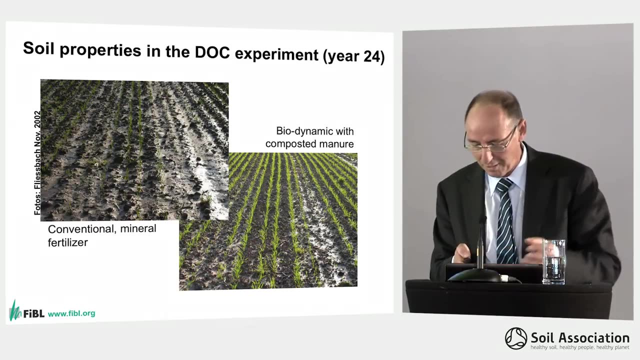 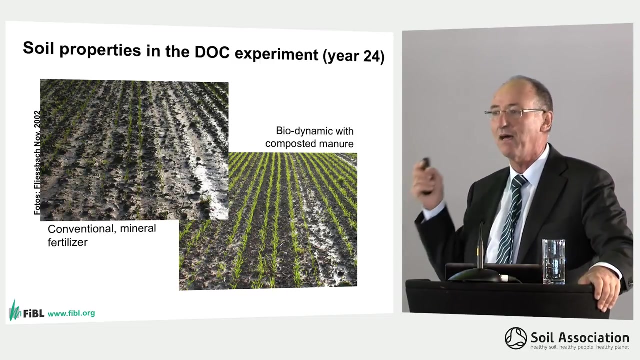 and here you have a surface, your professional storage of water and and, and the soil structure gets destroyed and you have a runoff of water into, into, into the, into into the streets and so on. so it is really a huge difference how soil biology can, what soil biology can do. 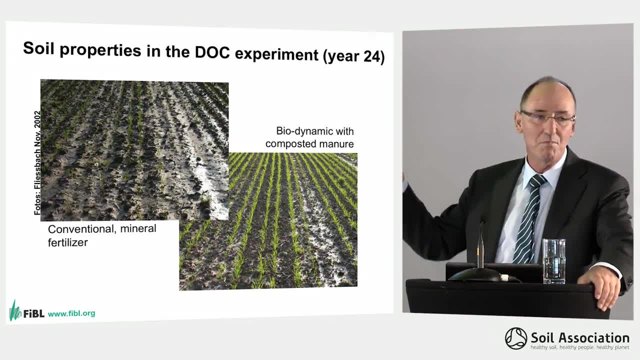 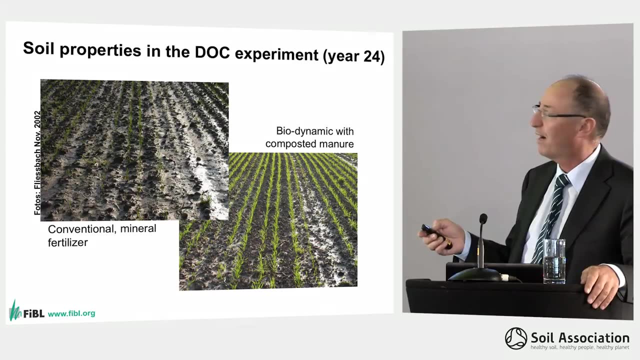 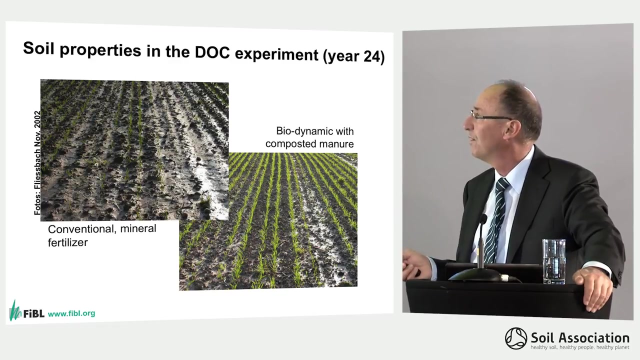 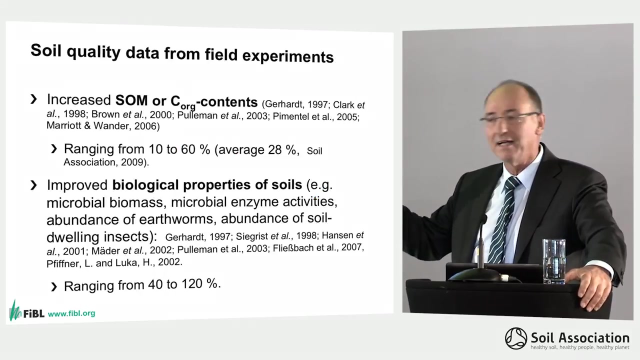 with soil structure and for me, this is the most important advantage of organic farming. we talk about drought resistance, drought resilience. we talk about climate change and this will position organic farming very high on the agenda. if we talk about adaptation to climate change and all what I showed here and i could show a 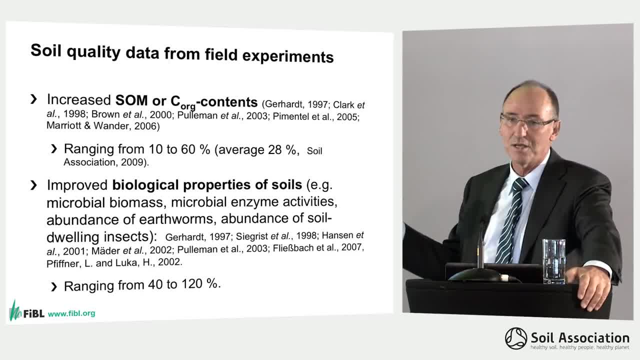 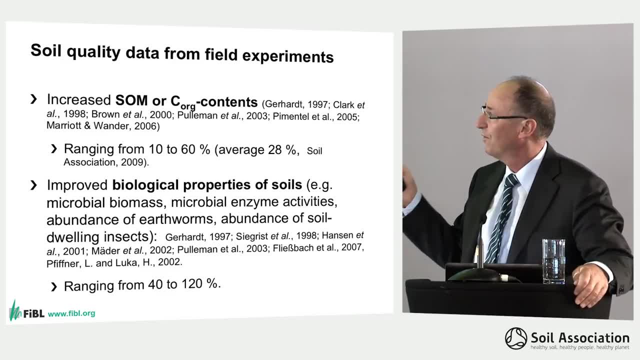 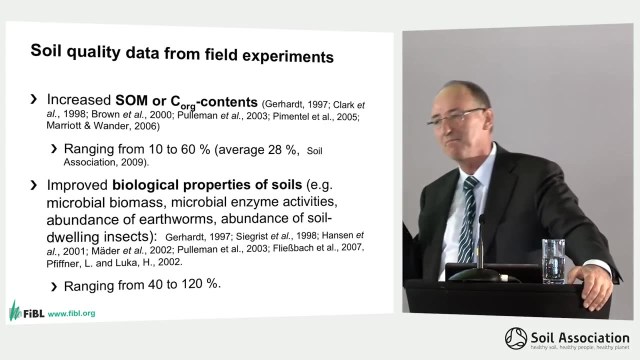 lot of results more because we didn't did a lot of PhD. we performed a lot of PhD studies on this very field trial, because many students are extremely interested and many universities want to cooperate with us for PhD studies. So I could show you hundreds and thousands of more results, but all what? 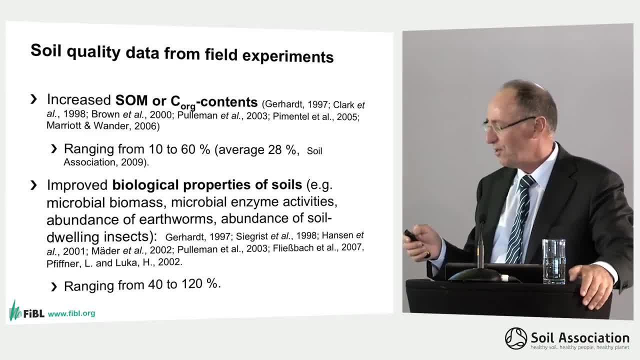 we measured in our DOC trial can also be shown with a lot of literature. For instance, increased soil, organic matter and CO contents in soil was shown by other studies already for a long time. Improved biological properties of organically managed soils is also shown, approved by many literature studies, and the difference between conventional and organic. 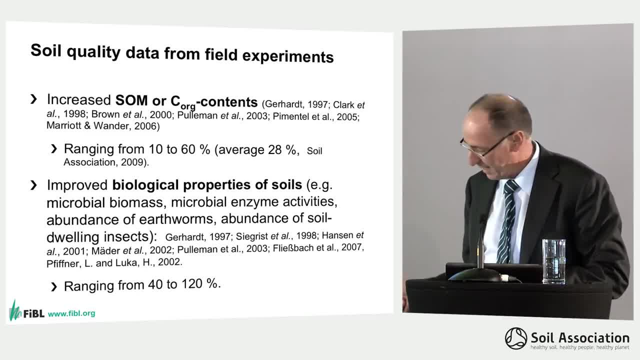 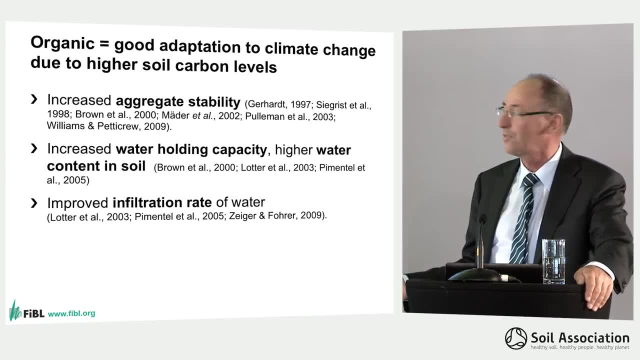 ranges between 40 to 120 percent. Also, the increased aggregate stability has been published by different authors. and the increased water holding capacity, higher water content in soil and improved infiltration rate of water. So everything is well known, well documented. we really have a strong basis for our claims that organic farming is really one of the 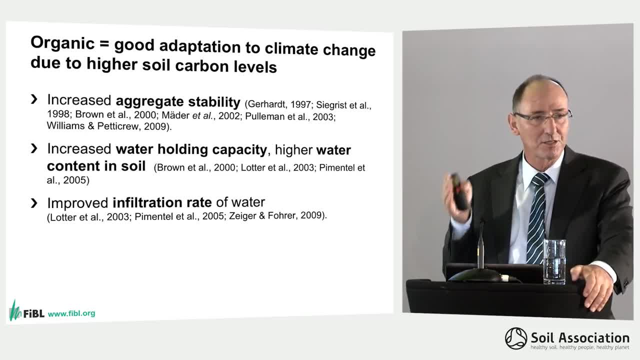 solutions for all our soil problems we have, And it's a productive solution. it's not an unproductive solution. so it is an ideal combination between soil, between food productivity and soil conservation, And I was very, very amazed that the results of this trial were very, very good. 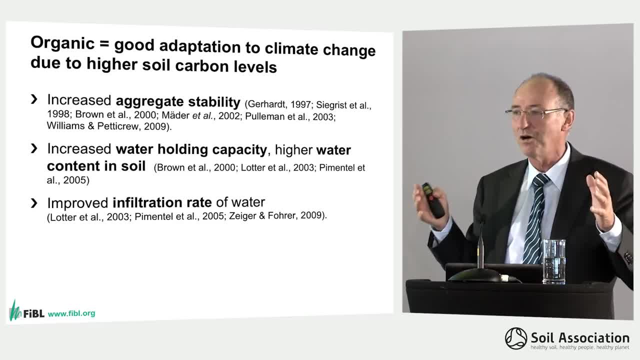 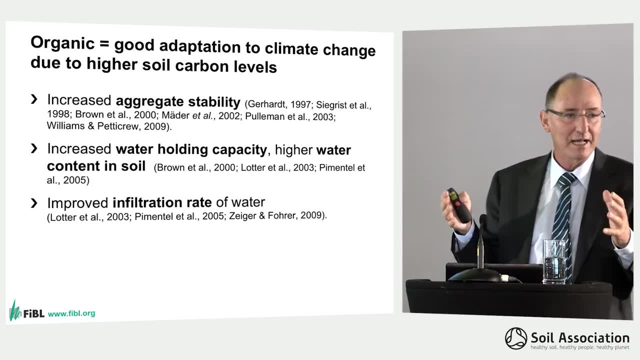 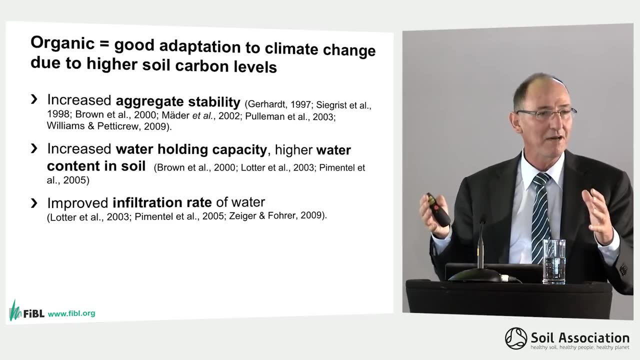 Last week, when the International Global Soil Week was in Berlin, that everybody was agreeing on that. we have a soil problem, but nobody knew the solution for the problems we have created with industrialized agriculture. But in the run of the week more and more people started to talk about organic farming. 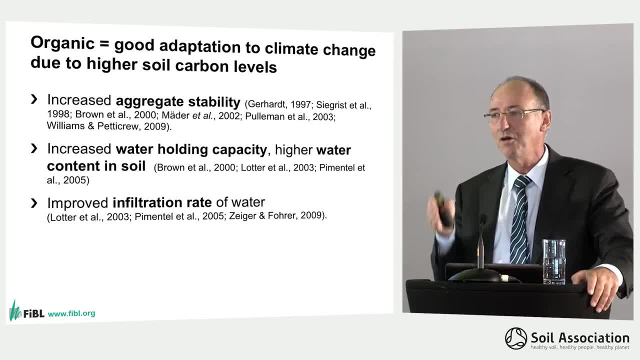 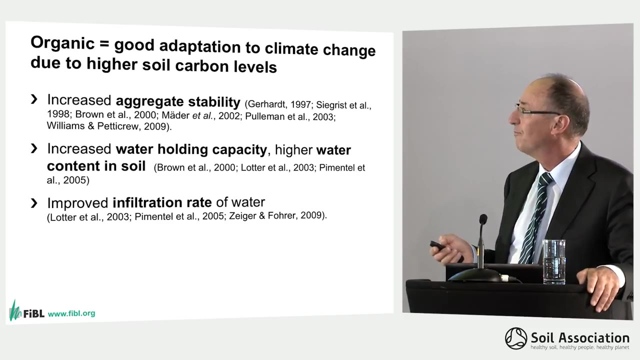 And it was really a hot issue at the Global Soil Week in Berlin that organic farming could offer solutions. So we will see 2015,, the year of the International Year of Soils, that we can push this agenda of organic farming. Now. a further question is: can we even have 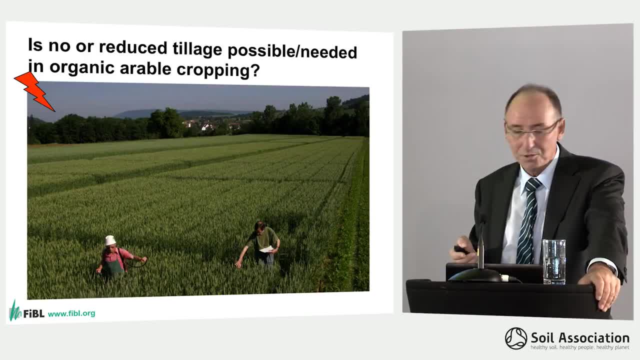 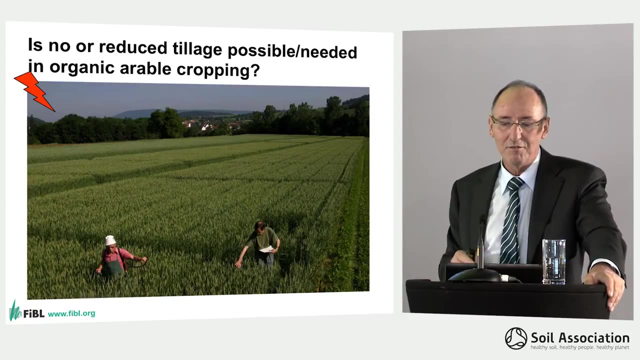 less tillage. Can we even do better? And we try to do that by combining reduced tillage systems with organic arable cropping, And you can see this. this is the research field which is at our institute in Switzerland, in the northern part of Switzerland. It's a heavy soil and you can see the field all. 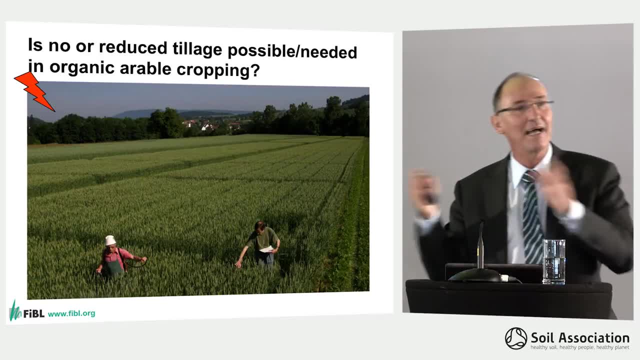 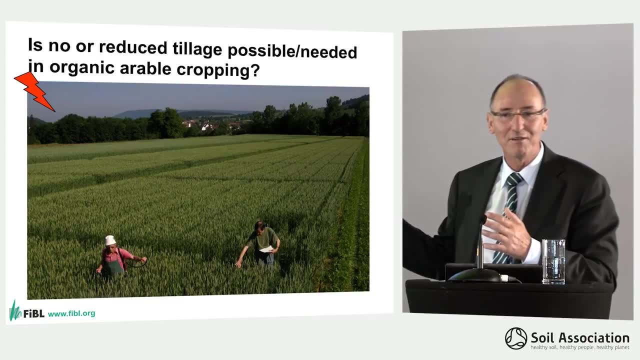 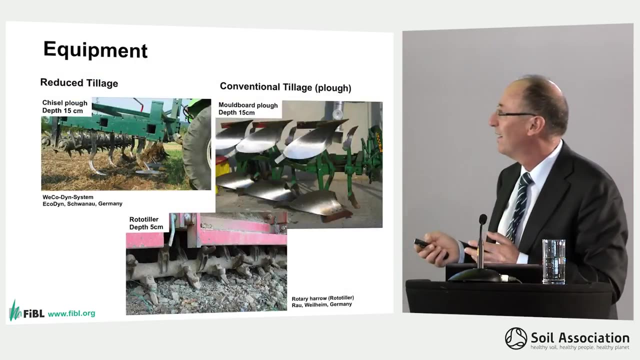 all the different treatments, reduced till and ploughed. everything looks still perfect here after 6-7 years. so we are not under with wheat, so we still perform well and that's how we perform the different systems. so we have a chiseled plough. 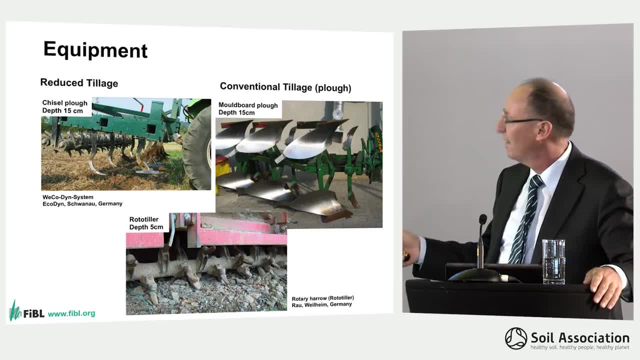 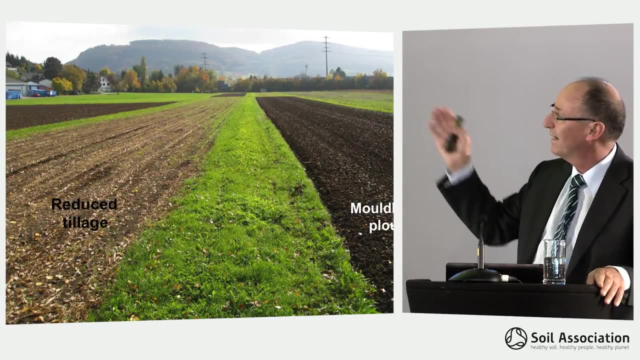 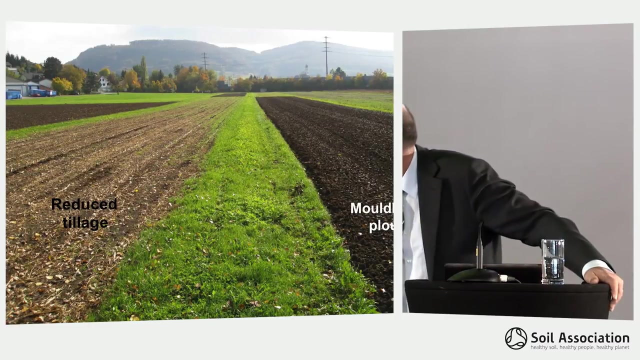 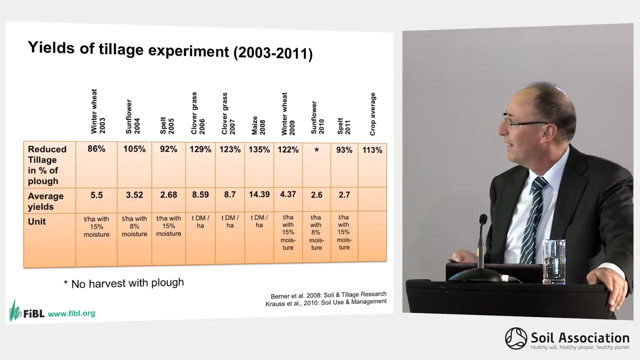 for the reduced system and we have a mouthboard plough for the conventional system and we also use rototiller. you can see here the different systems. so this is the ploughed one and this is the reduced tillage one. and to be short, if we look at the yields of the reduced tillage system. it started with winter wheat in 2003 with 86% of the yield of the ploughed one. it's only convention, it's only organic. comparing plough versus reduced tillage, the sunflower next year was: 105, the yield was spelt 92%. the clover grass two year lay was 129, 123 and then the maize, following this lay was 135. so the longer the system run, the reduced tillage, the better the yields became. and the winter wheat. 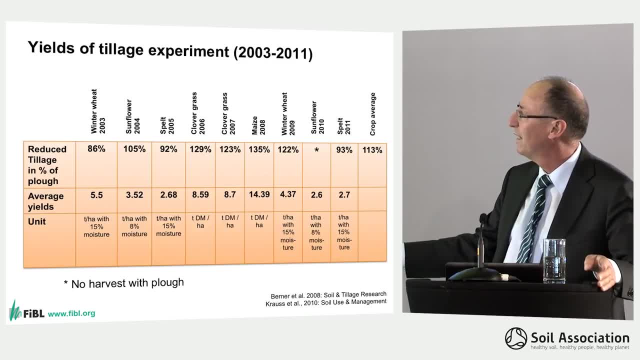 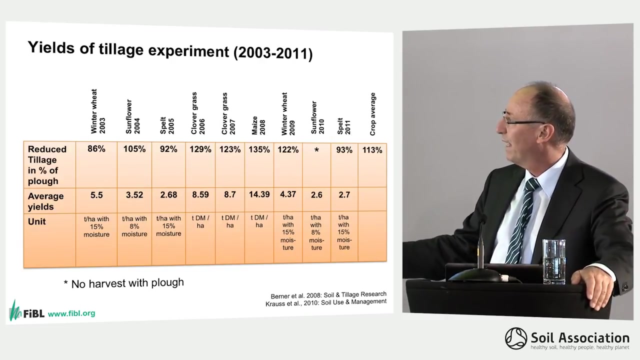 in 2009, 122% and here, unfortunately, 2020. with sunflower, we harvested only in the reduced till system and we didn't harvest in the ploughed system because we couldn't harvest. it failed completely and spelt again. 93% in 2011. 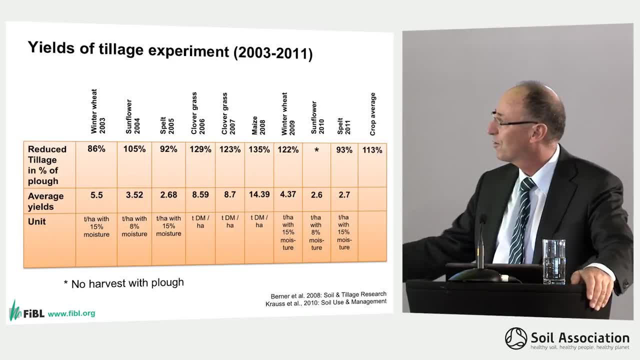 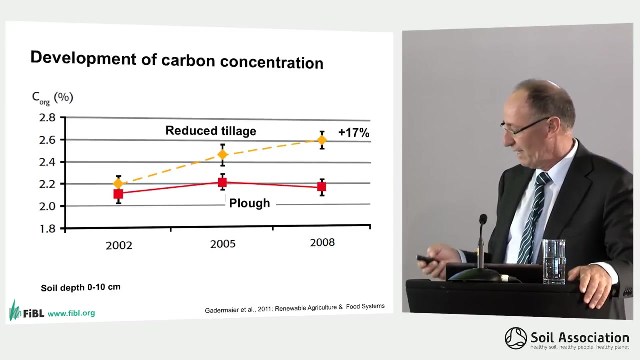 so over more than one crop rotation- it was from 2003 to 2011- the crop average of all crops was 13% in favor of the ploughed plots. so obviously it's quite. it's feasible to harvest more with reduced tillage. very. 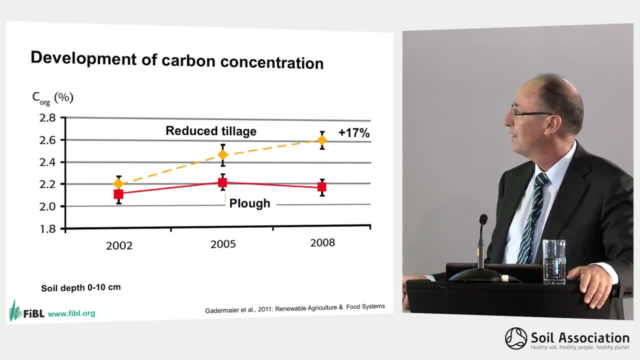 interesting, the carbon concentration in the upper ground was increased by reduced tillage by 17%. this was on soil depth between 0 and 10 cm and between 10 and 20 cm. the difference was 7% and we already see that, thanks to the 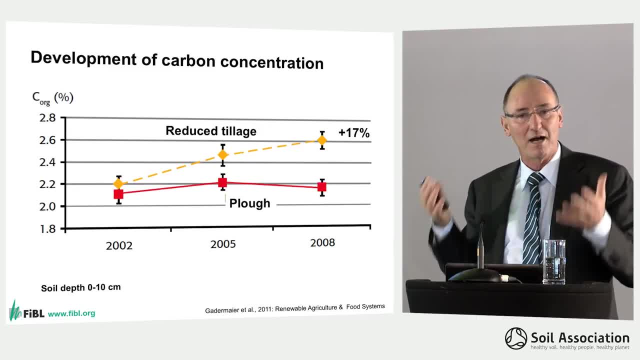 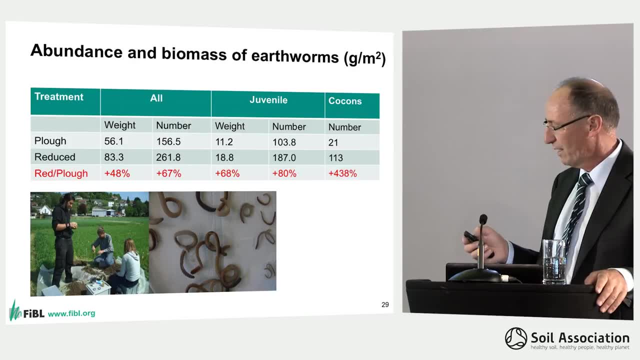 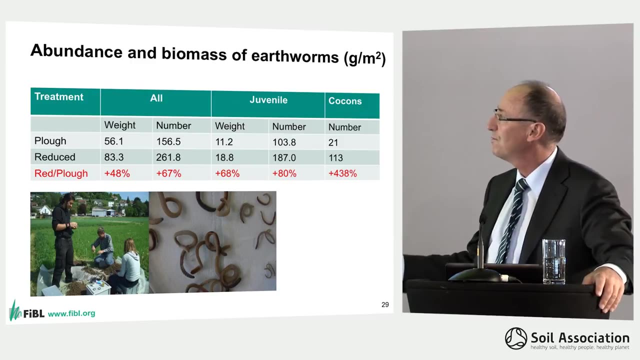 earthworms. the increase of carbon goes down in the soil profile. so a very important number information to give is the abundance and biomass of earthworms measured in gram per square meter. so we can see that over all earthworms the weight increased in the reduced tillage. 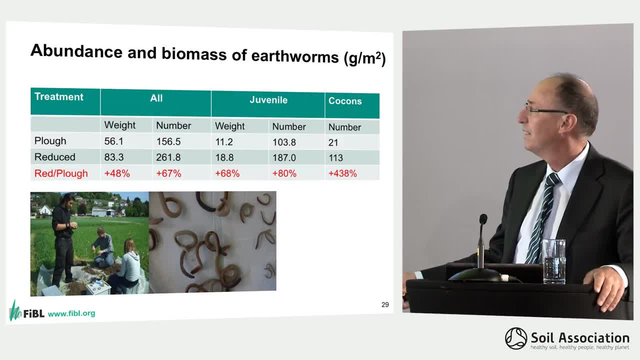 system by 48% and the number of animals increased by 67%: juvenile, young earthworms, 68 in favor of the reduced tillage system, and the number went up by 80% in favor of the reduced system. and look at the cocoons. 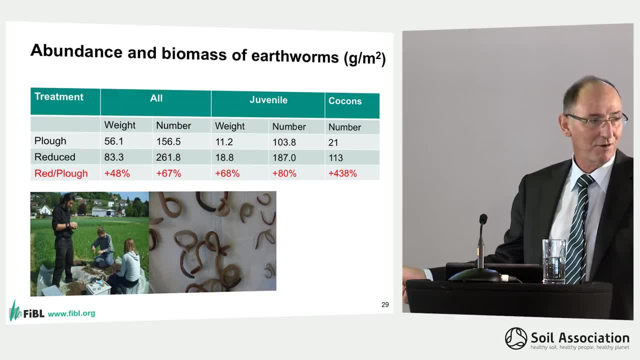 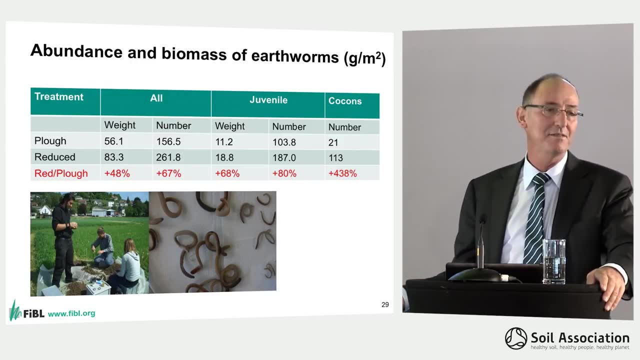 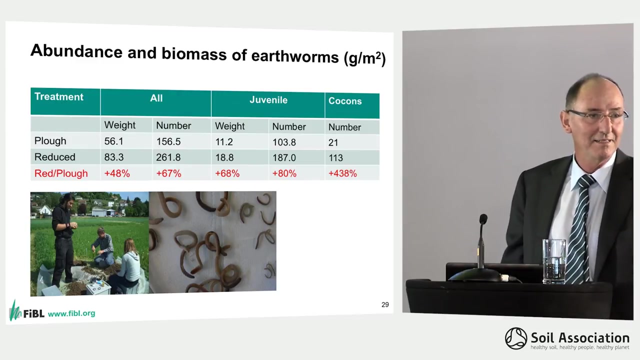 which are the eggs of the earthworms. so here we have an increase of 438% in the reduced tillage system. so you can really. so this reduced tillage system, without using GMO, without using glyphosate, without using nitrogen fertilizer, can be combined with organic and it is 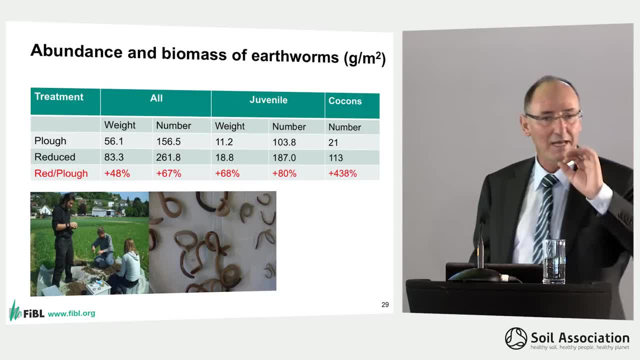 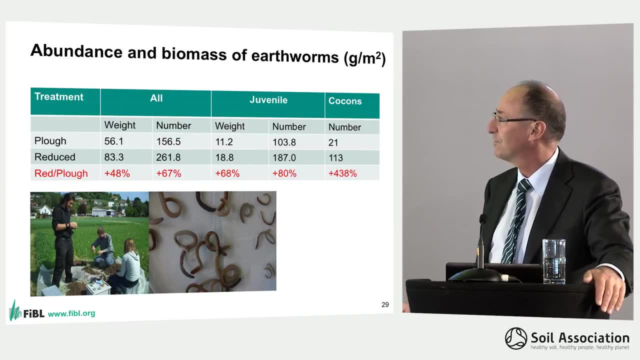 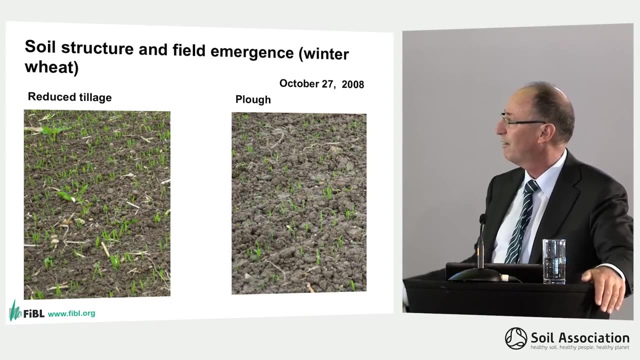 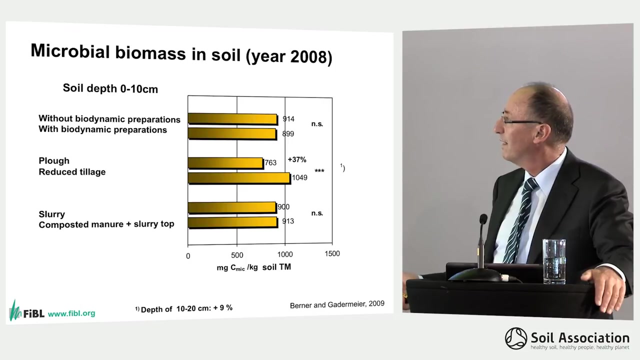 extremely successful farming system. we have to develop that further and farmers have to become familiar with that kind of system again here. field emergence for winter wheat reduced till very good field emergence and plough- it is much weaker. soil micro biological mass was also increased by reduced tillage. 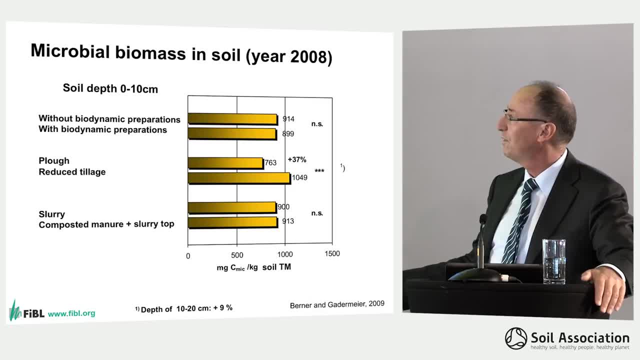 considerably. it was not increased by whether we used biodynamic preparations or not, because we not only have the difference between plough and reduced tillage, we also have the difference between slurry and compost manures and top fertilization with slurry and also with and without. 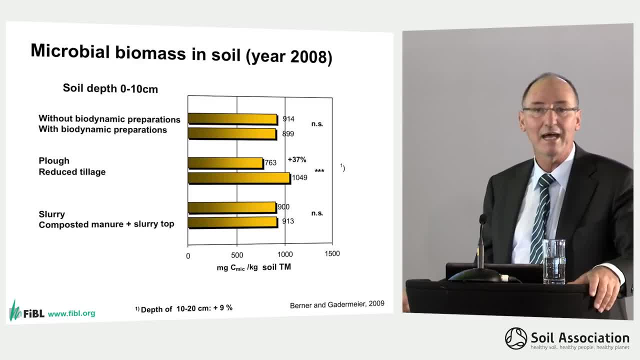 biodynamic preparation, because many biodynamic farmers tell us that biodynamic preparations are very helpful in converting from ploughing to reduced till. but we didn't see any difference of that. but there is a huge difference between plough and reduced tillage. it's much bigger, the soil. 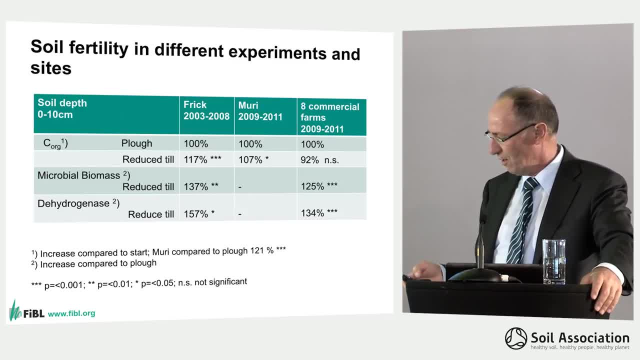 biomass here, and only to show that it is not only one site we produce results from, so this it's also other sites. this is the experimental sites I already showed. we have another one and we have eight commercial farms, farmers who practice this kind of reduced tillage. 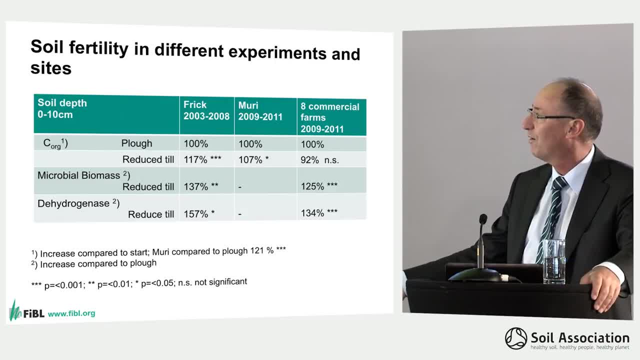 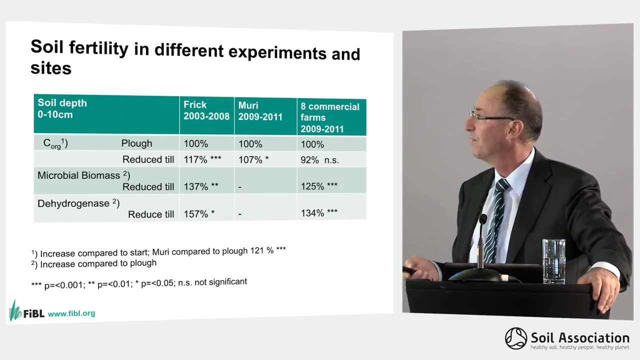 system. and you can see for Sea Org, microbial biomass and dehydrogenase that with reduced tillage we always have increase with reduced tillage, so meaning that soil fertility is really heavily profiting from that kind of farming system. and finally, this is about eco functional. 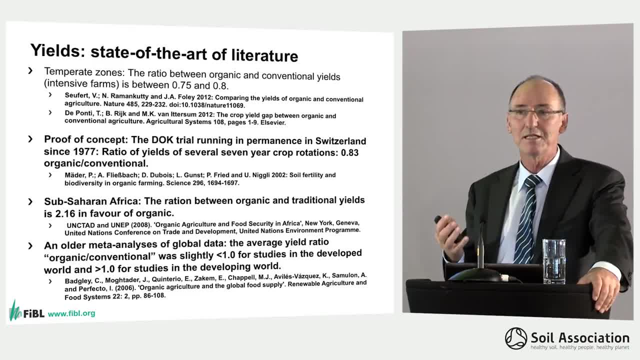 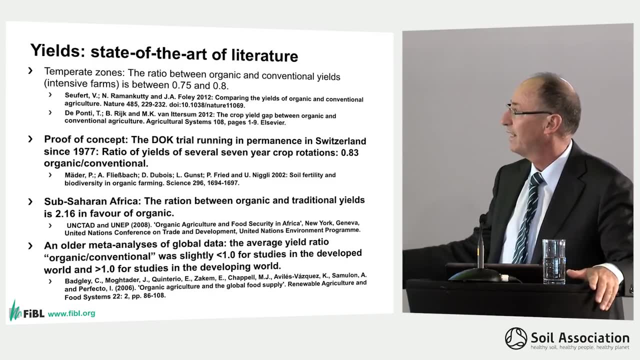 intensification because we have to use soil fertility to increase our yields. we are much criticized of not producing enough to feed the world and fortunately there is a lot of data available from different meta studies, but also from long term field trials, from case studies done by in Africa. 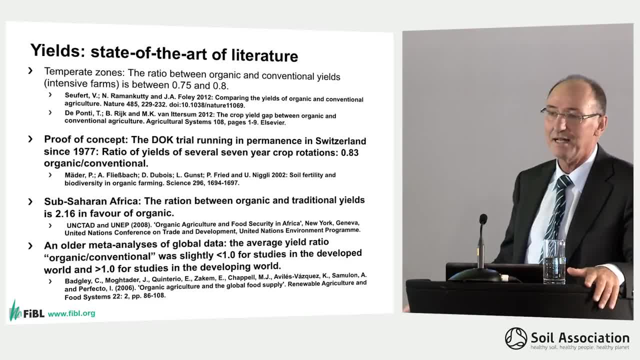 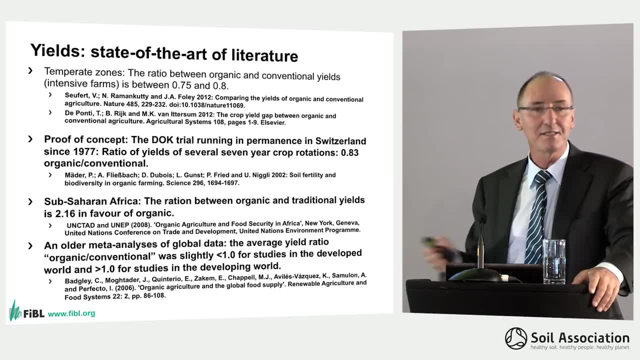 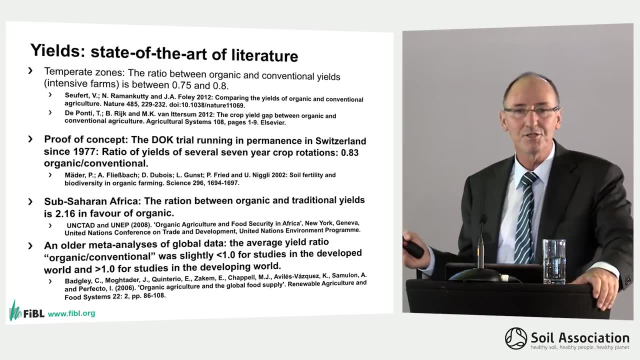 and also by other meta analysis from the United States, that the yield of organic is somewhere between 70 or 80% of that of conventional, and this is far higher than those campaigners against organic farming always claim, because they cite figures like 50% yields only. so 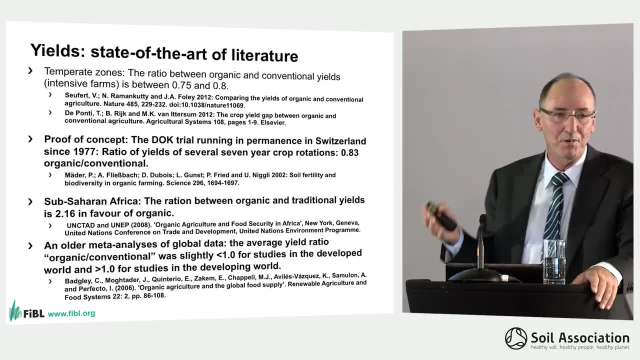 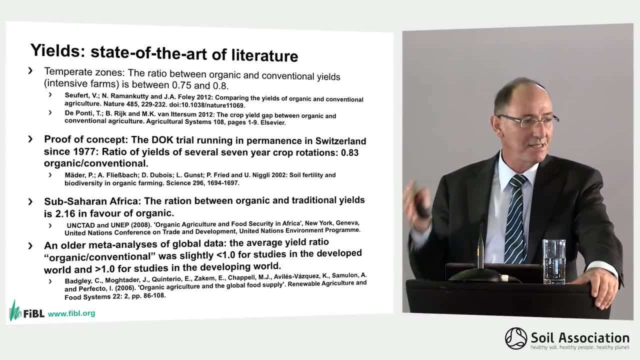 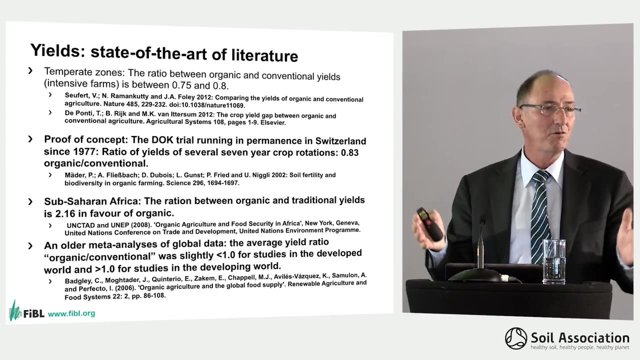 the worst case we produce might be about 30 to 40% less yields in certain circumstances, but all what we harvest less than conventional farmers is much below the food we waste 30 to 40%. so we are much better than that. so for me the solution 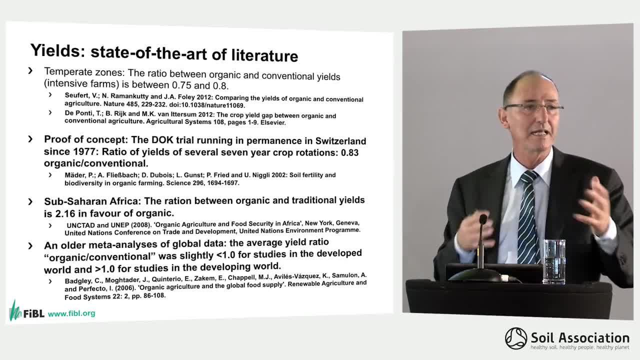 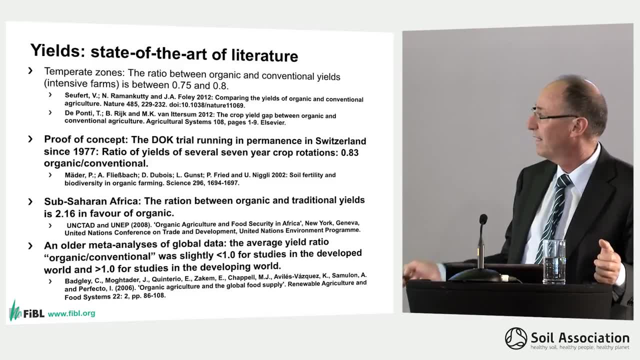 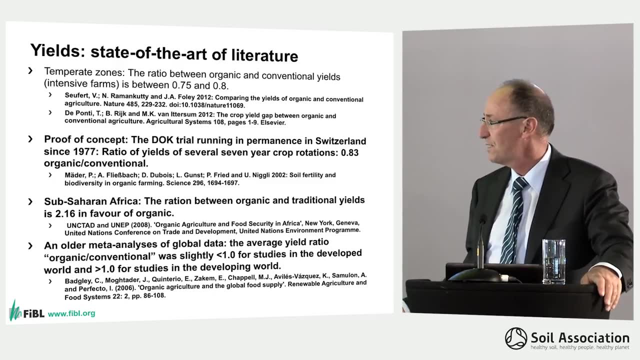 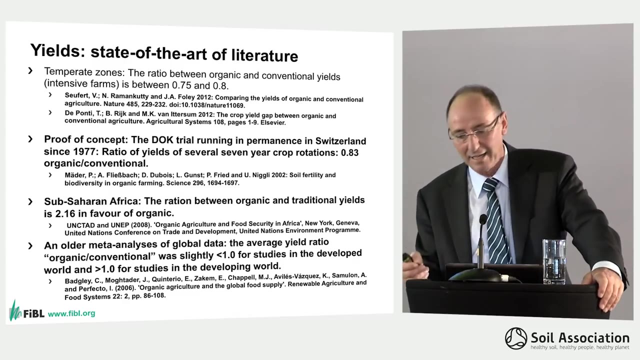 the question whether we produce enough or not cannot be answered in an isolated way, without an analysis, and many of the studies from sub-Saharan Africa, where food is really needed, show- and this is thanks to Heinz and Pretty- show that organic farming can double or even triple the yields of. 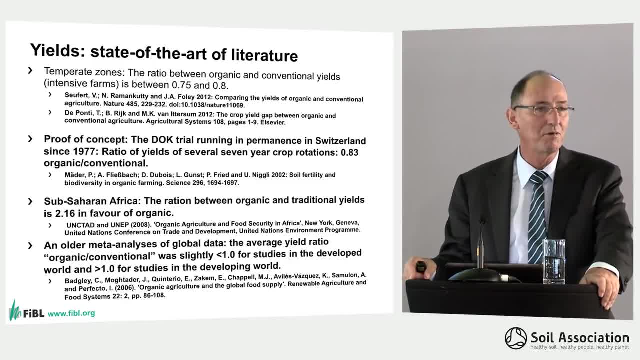 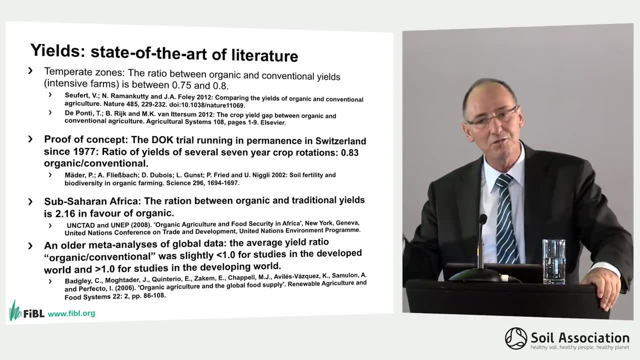 farmers, and this is the most important information, because it can improve yields, it can improve livelihoods in sub-Saharan Africa, and this is a very important information. but nonetheless, we devoted ourselves to produce more in our scientific concepts, and this is all about ecological or eco-functional intensification. so to 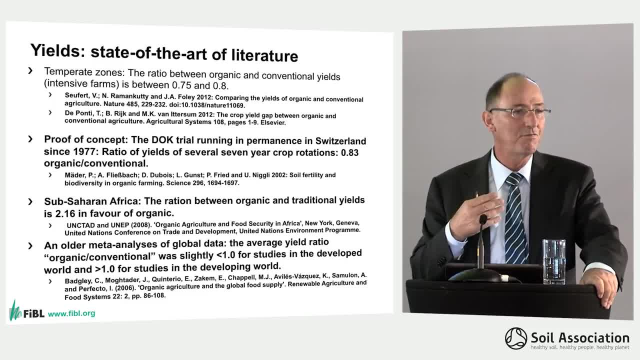 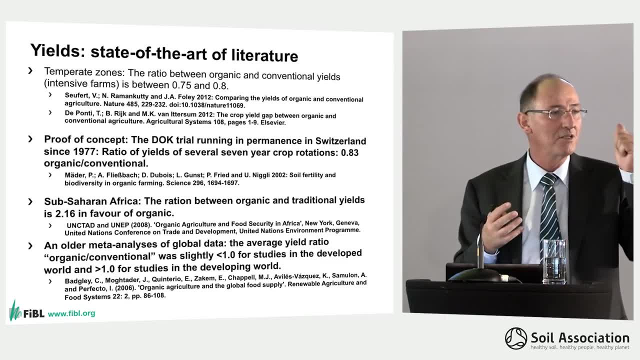 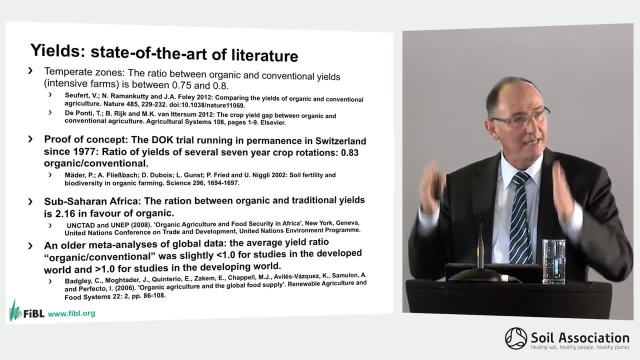 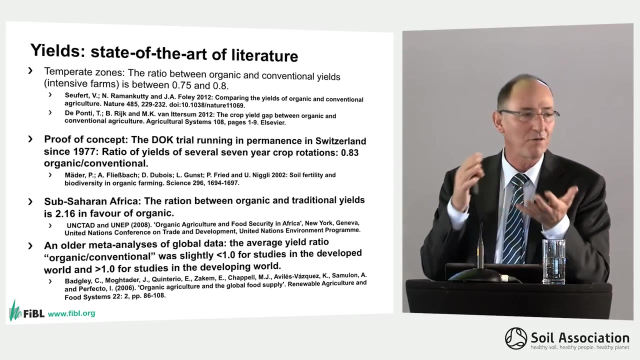 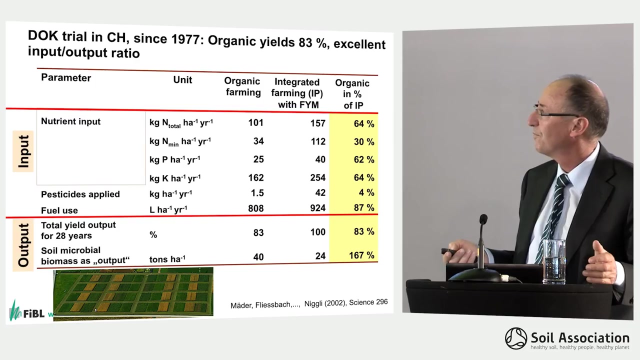 produce more with eco, with the functions of our ecosystems, and the functions of our ecosystems are soil fertility, for instance, are biodiversity, and so on and so on, and I think it's possible to increase the yield, to diminish the yield difference with organic systems, via utilizing ecosystem functions. 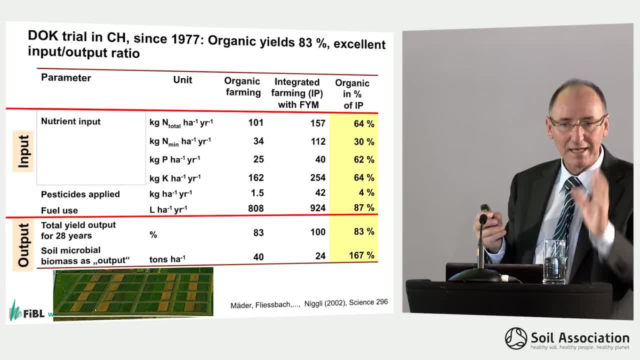 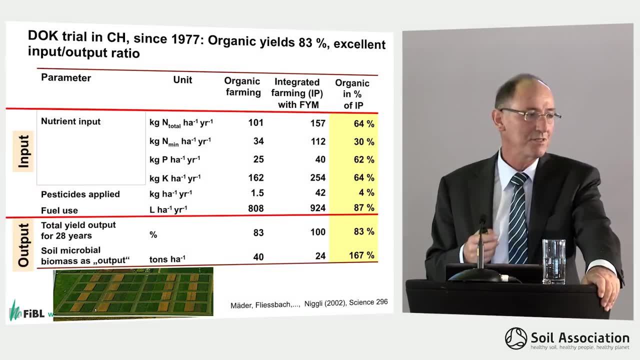 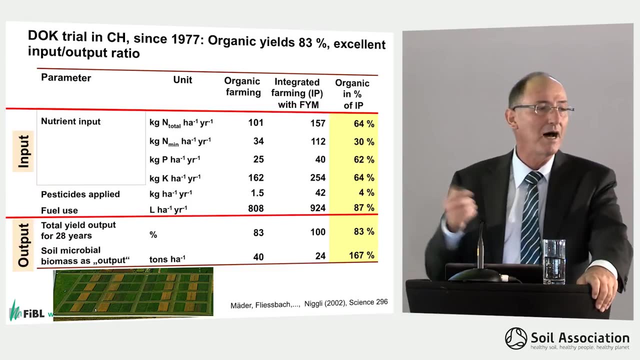 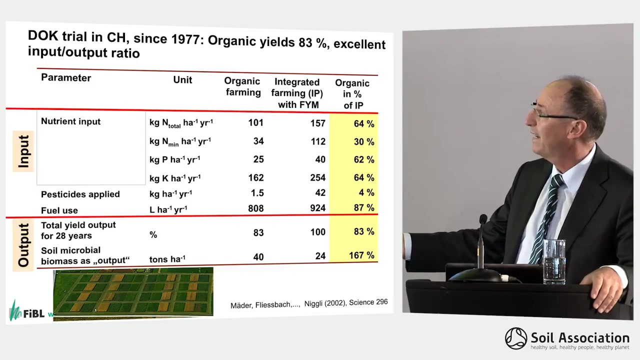 and another question we have to talk about is efficiency and sufficiency and efficiency. everybody is talking about efficiency: making more out of less. this is the Syngenta and the Monsanto slogan, and but we already do that. if you look again at this: dog trials since 1977: organic. yields over all these long periods of more than 30 years. organic yields are 83% of the conventional ones. and look at the input. the input is for pesticides: 4% compared to conventional farming system. for mineralized nitrogen, 30%, for total nitrogen only 64%. for phosphorus 62%, for potassium 64%. so, looking at input and output, organic is already the most efficient farming system and if you take into consideration also the soil, microbial biomass building, and this is in a way, also an output. it is an output produced on the ground. 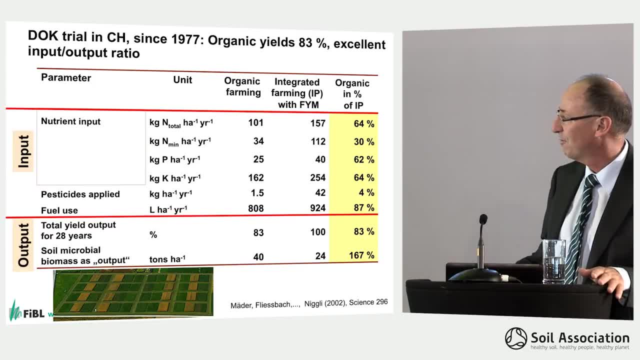 and here the efficiency of organic is 167%, so fantastically efficient organic farming. we don't have to hide away our success stories. we are good, we are efficient and this is very important. and if you look, for instance, at phosphorus, which is restricted, the chemical. 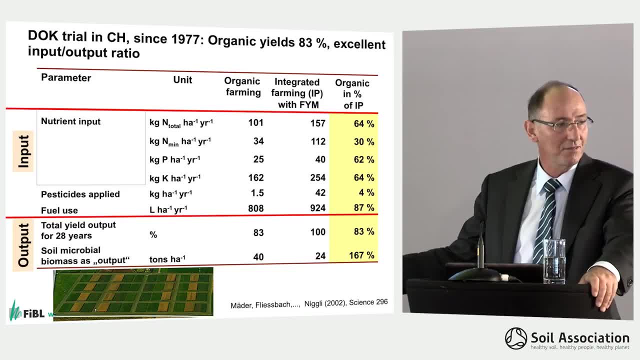 industry. they talk about another 300 years for mining. critical scientists talk about 100 years for mining still left. but if you look at phosphorus, this is very efficient use of phosphorus compared to the output. most of this phosphorus is from recycling, from livestock, so 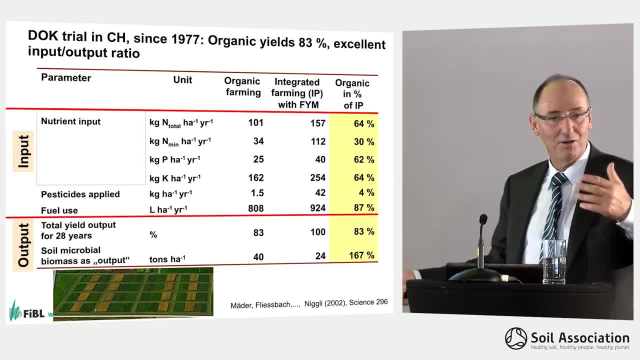 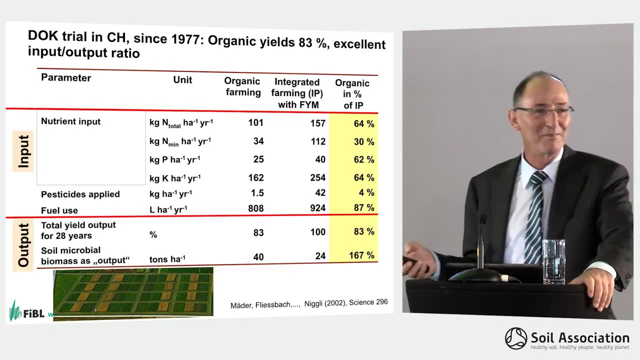 this is, in a way, what we called sufficiency. sometimes English words are very complicated- sufficiency meaning that we keep. we use limited resources in an efficient way, but we also recycle it. this means sufficiency with our way of farming. we can keep on farming another 600. 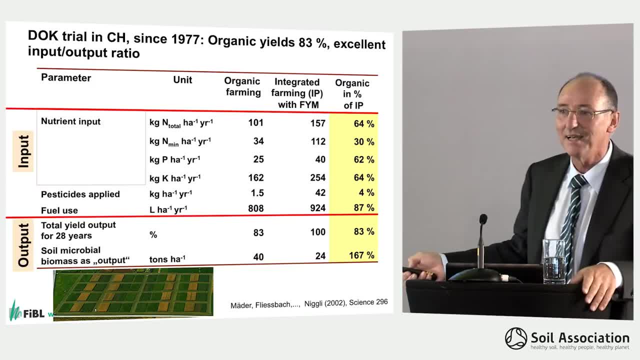 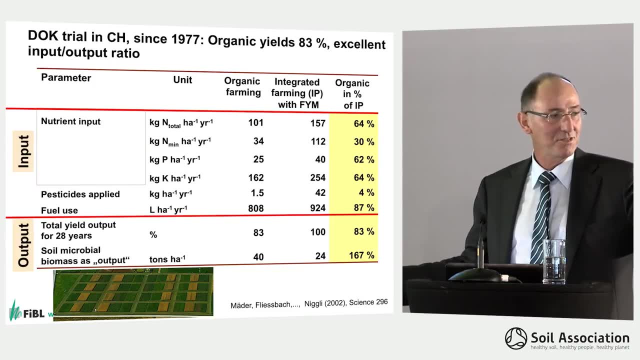 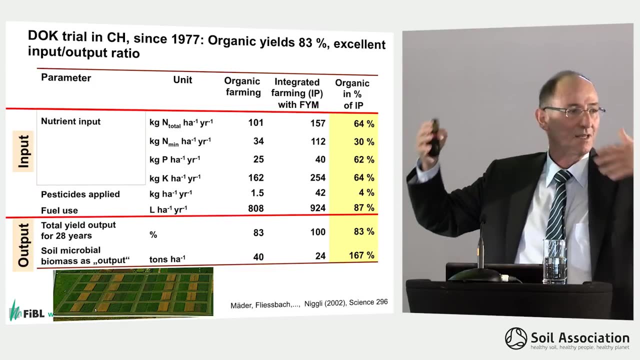 or 1000 years, not only 300 like the industry says. but still we are not there where we want to be. Helen mentioned it. we have to close also the big circles from human waste and so on. so this will be the next challenges we will face. 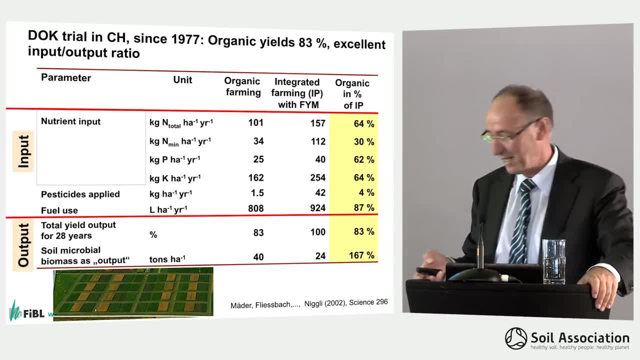 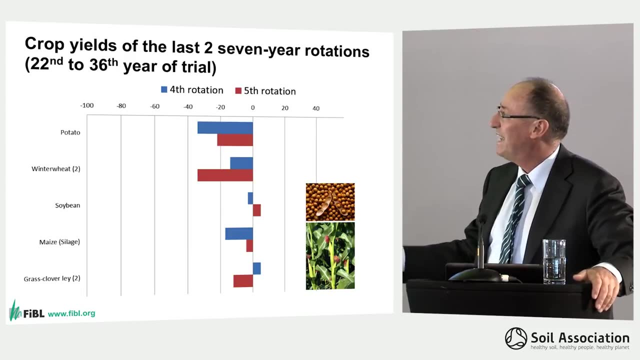 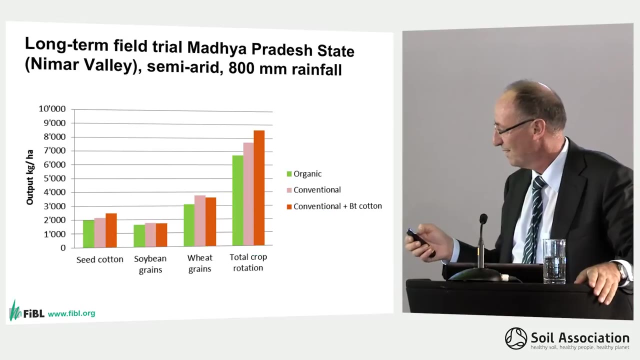 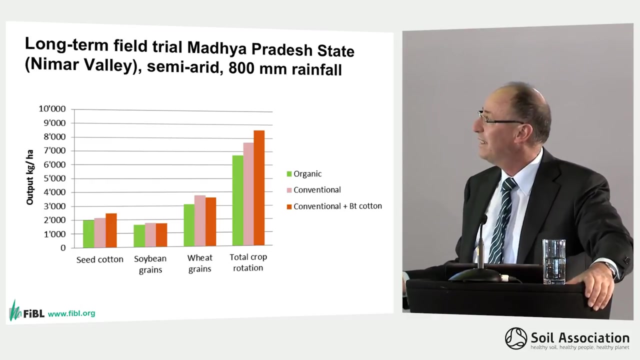 and this will keep us busy for a long time, fortunately, because that's one reason that scientists will still be needed in the next decades, also about yields. basically, we have not yet generated as many scientific results from our tropical soil experiments, but at least I can show you some. this is in: 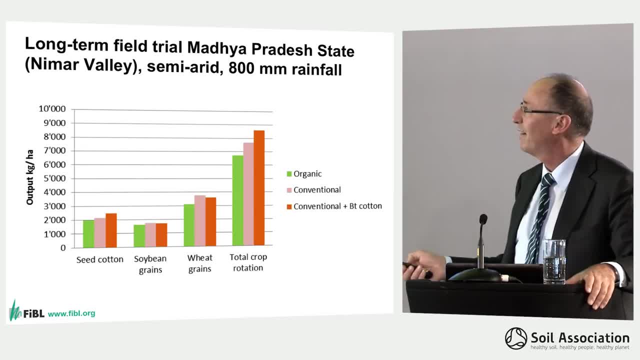 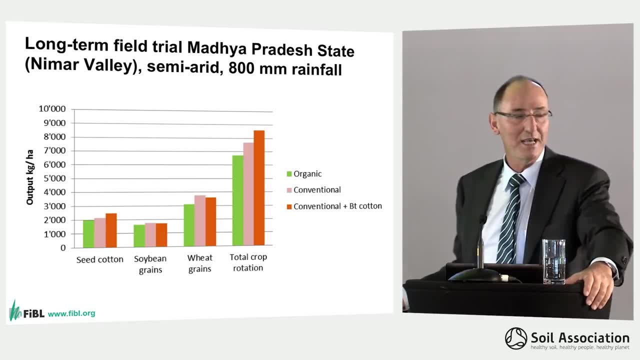 Madhya Pradesh state semi-arid zone, where we compared organic, conventional and conventional plus GMO BT cotton. we didn't want to be criticized that we didn't use the latest technology. that's why we planted BT cotton in an organic field trial and you can see here the difference already of two crop rotations, the yields. for seed cotton the differences are not as big. the conventional BT cotton system is the best one. for soybean it's almost no difference, for wheat grains it's also only a small difference and for the whole crop rotation the yields are highest. 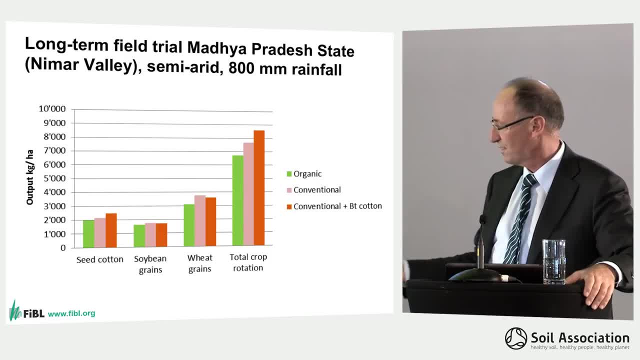 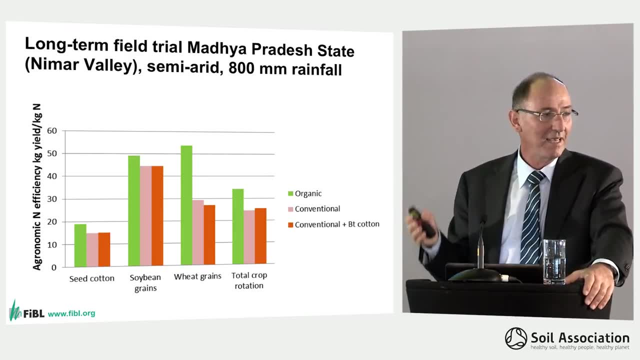 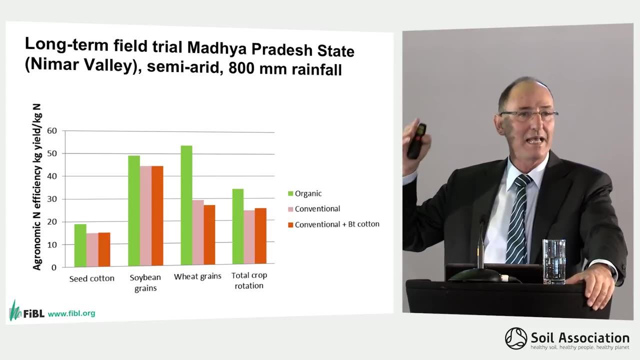 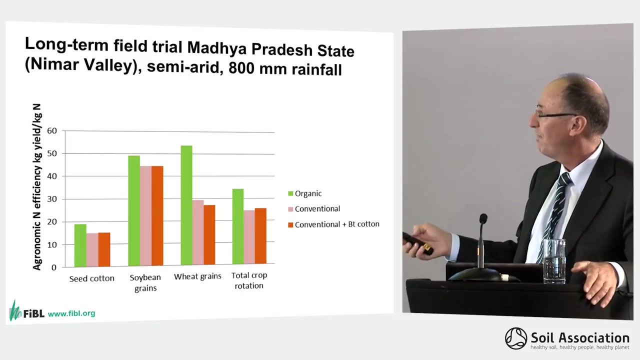 in the conventional and BT cotton system. but again, if you look at agronomic N efficiency- input, output, because the conventional organic yields have been produced with less nitrogen, much less nitrogen than the conventional. if you look at efficiency, then you can see that seed cotton the most efficient Newton. 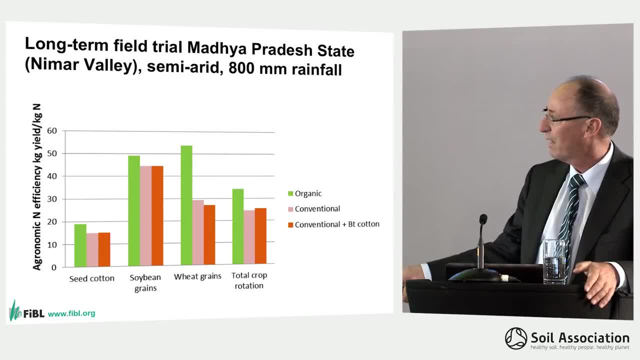 efficient system is the organic one by far, and also for soybean organic is by far the most efficient one. for wheat grains, organic is even terribly efficient and over the whole crop rotation organic remains the most efficient nitrogen using farming system and the BT cotton, although everybody thinks. 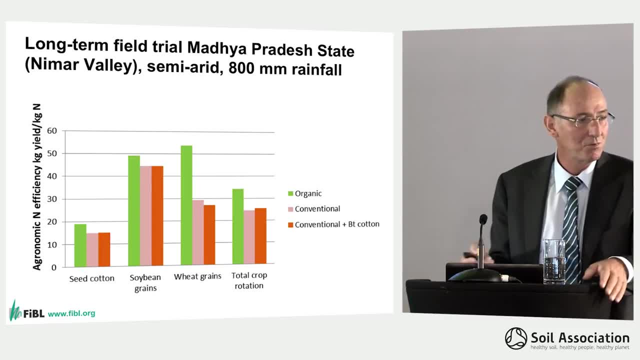 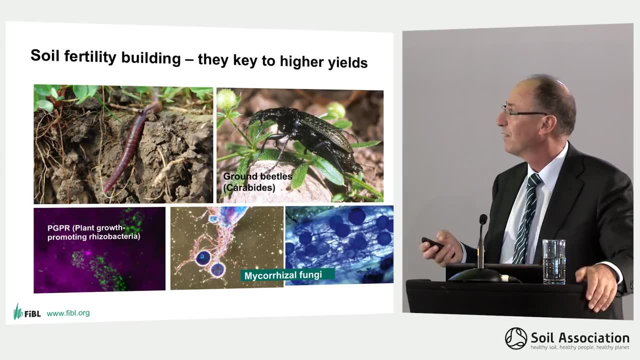 that it is the solution doesn't really contribute to the solution of that problem. so soil fertility building for me, is the key to higher yields, and we have so many friends in our soils and at the moment many scientists work on this plant growth promoting rhizobacteria. 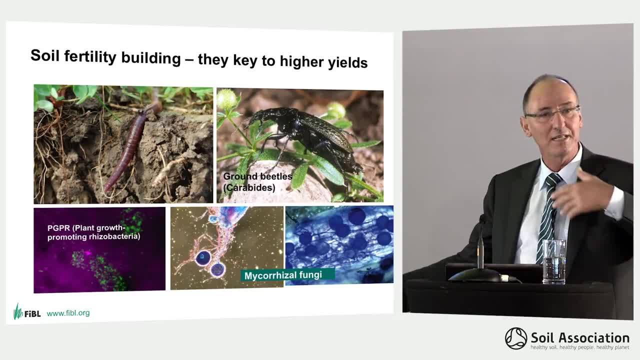 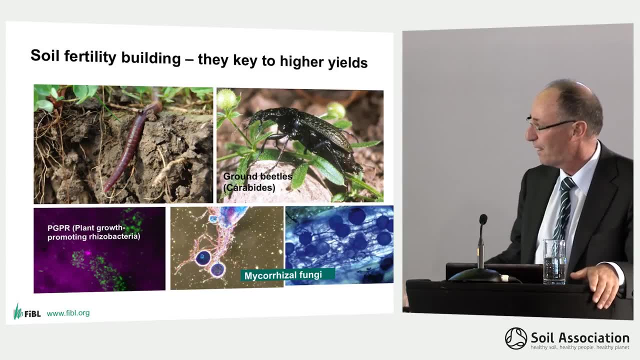 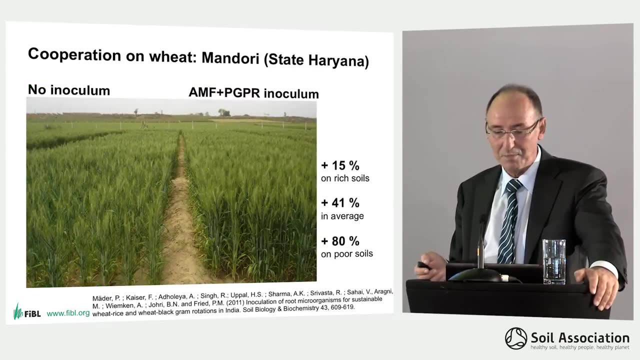 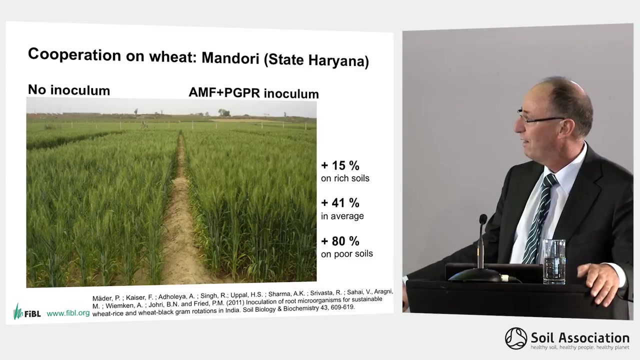 which are added to soils and which can increase the access to phosphorus and other nutrient elements. and also, many people work on mycorrhizae. only one picture from Mandhuri, the Haryana state in India. this is wheat without inoculum and it is. 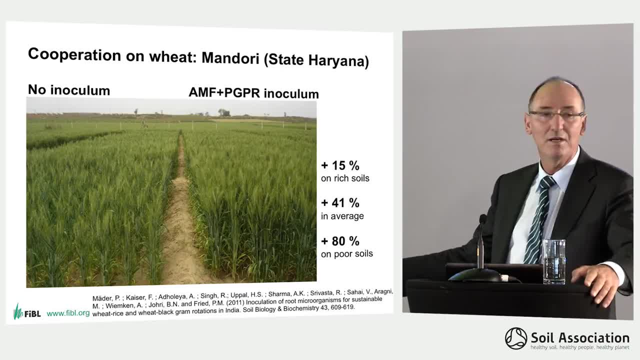 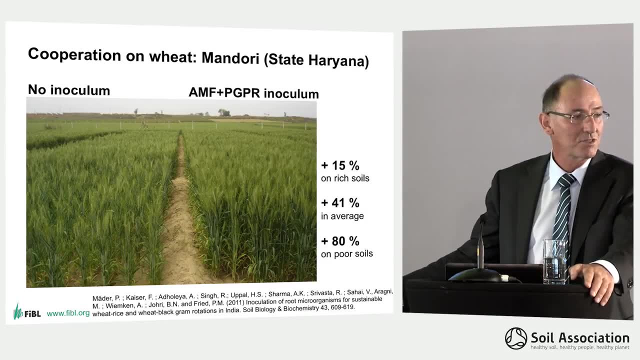 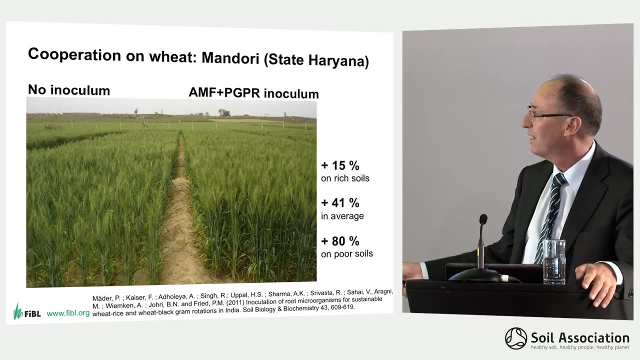 mycorrhizae and PGPR inoculum, a mixture, and you can see here the density of the wheat thanks to the inoculum is much bigger than without this inoculum and you can see, on rich soils the yield increase is 15% in average. of all 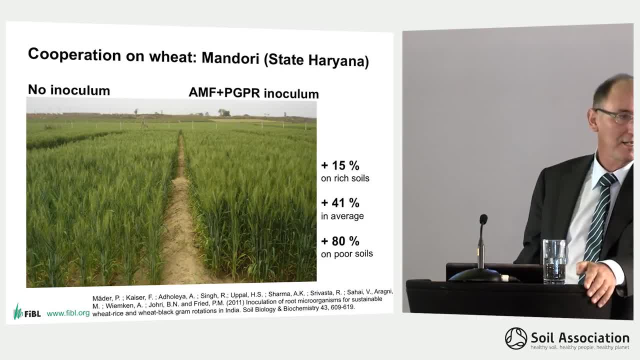 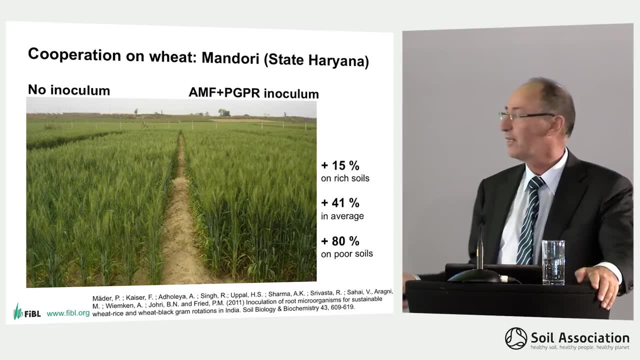 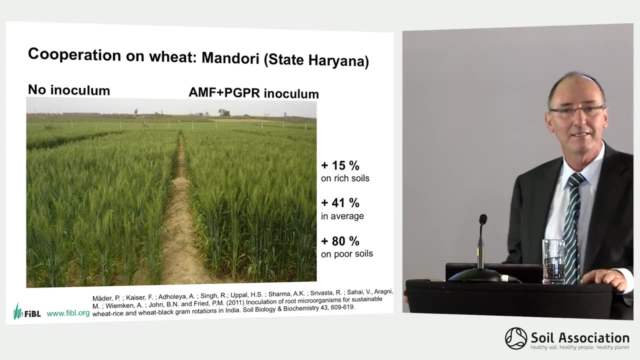 sites in India it is 41%, and on poor soils it is 40%, and this is exactly about eco-functional intensification. there is a new consortium working on exactly that, that approach, using it also for temperate zones. so I think this is really the way forward. 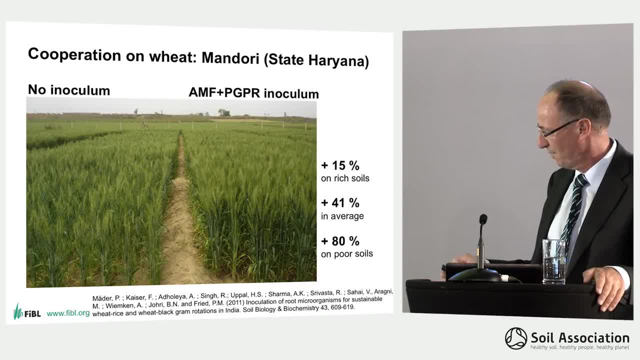 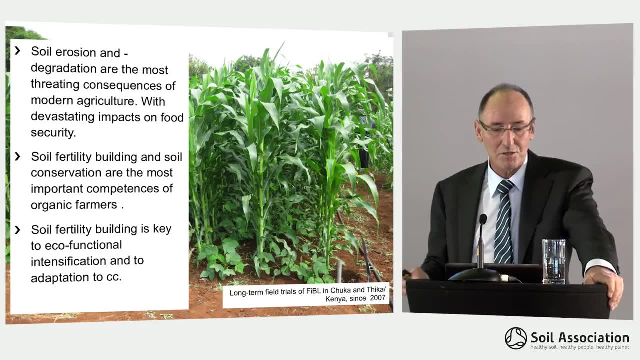 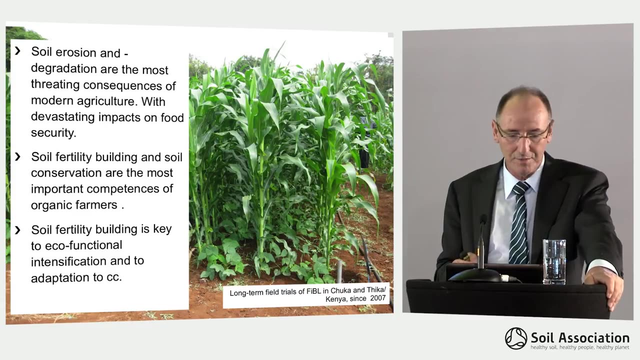 also for increasing yields. coming to the conclusions, soil erosion and degradation are the most threatening consequences of modern agriculture, with devastating impacts on food security. soil fertility, building and soil conservation are the most important competencies of organic farming. we can improve. that was shown. we can still improve. 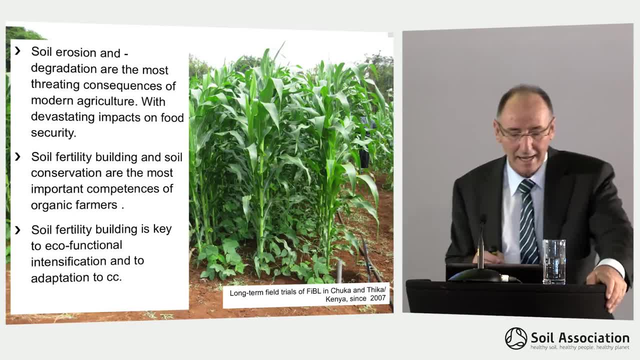 and soil fertility building is key to eco-functional intensification. adaptation to climate change. thanks a lot for your patience.